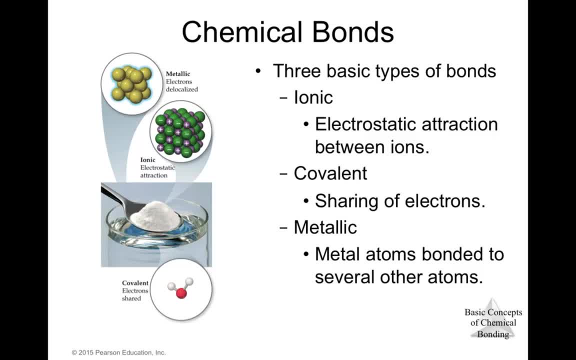 these three types of bonds by thinking about the simple act of using a stainless steel spoon to add table salt to a glass of water. Table salt is sodium chloride. This one, sodium chloride, is right here, And the structure is held together by ionic bonds which are due to the electrostatic 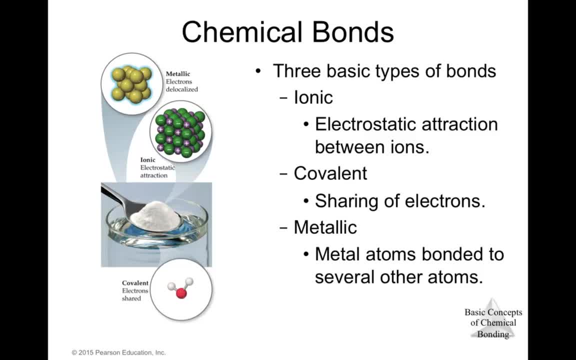 attraction between oppositely charged ions. The water that is in the glass mainly is H2O molecules. The hydrogen and oxygen atoms, as we can see here and we mentioned before, the red spheres are oxygen, the white are hydrogens. those atoms are bonded to one another. 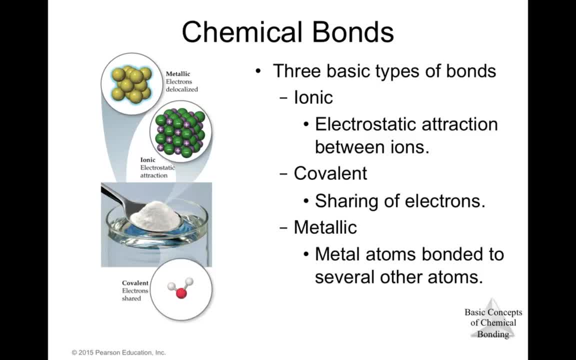 through covalent bonds. In other hand, the spoon consists mainly of iron metal, in which iron atoms are connected to one another via metallic bonds which are formed by electrons that are relatively free to move through the metal. These different substances- sodium, chloride, water and also 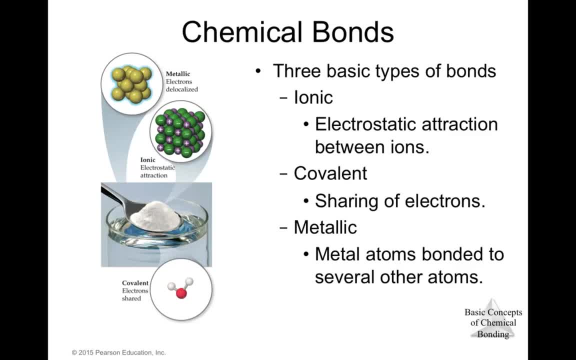 the iron metal behave in a similar way. The water that is in the glass mainly is H2O. The hydrogen atoms, as we can see here, are bonded to one another through covalent bonds. These different substances- sodium chloride- 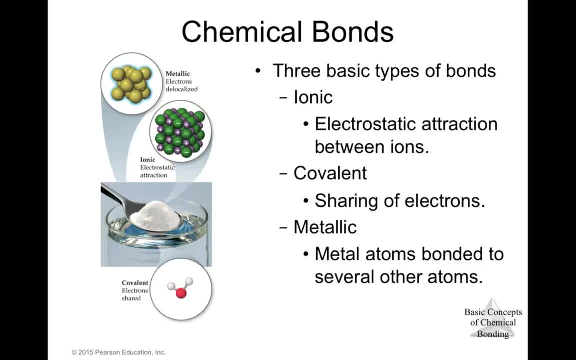 often behave as they do because of the way in which their constituent atoms are connected to one another. For example, sodium chloride readily dissolves in water, but iron metal does not. What determines the types of bonding in any substance? How do the characteristics of these 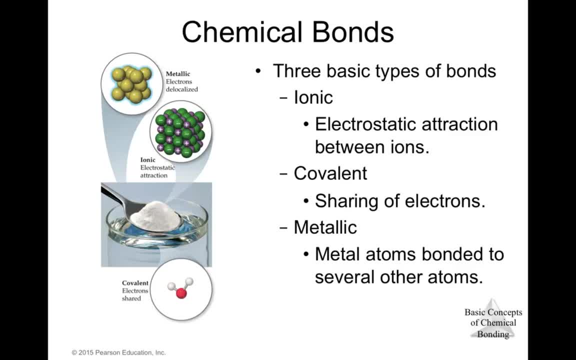 bonds give rise to different physical and chemical properties. The keys to answering the first questions are founded in the electronic structures of the atoms involved, discussed in chapter 6 and 7.. In this chapter and the next, we examine the relationship between the electronic structure of atoms and the ionic and 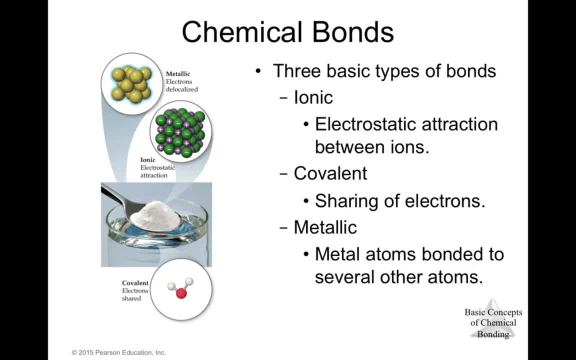 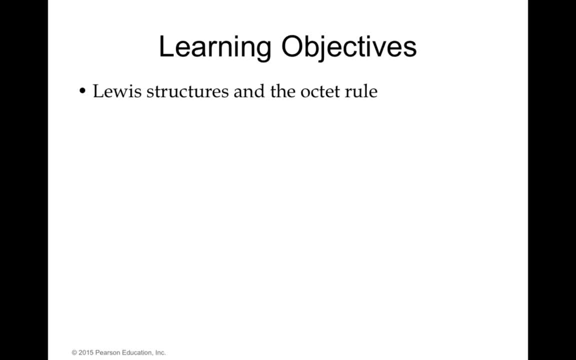 covalent chemical bonds that they form. So the learning objectives for this chapters are the: at the end of this we're gonna know how to draw structures and we're gonna learn also the active rule. We'll be able to distinguish between ionic and covalent bonding Also. 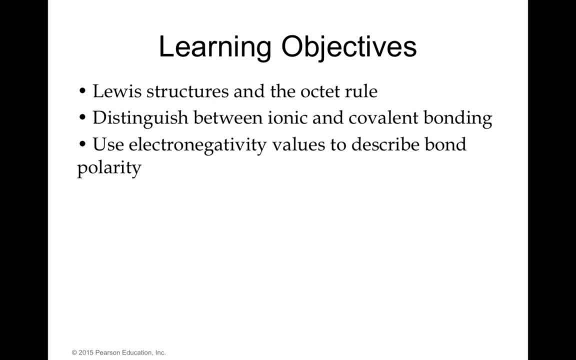 we'll be able to use electronegativity values to describe bond polarity. We'll describe also the localazide bonding and use resonance structure to represent the localized bonding. Also we'll determine the formal charge on atoms in a covalent structure and finally we'll talk about the relative or relate bonds. 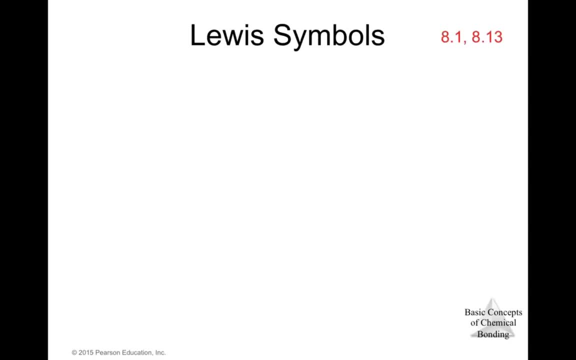 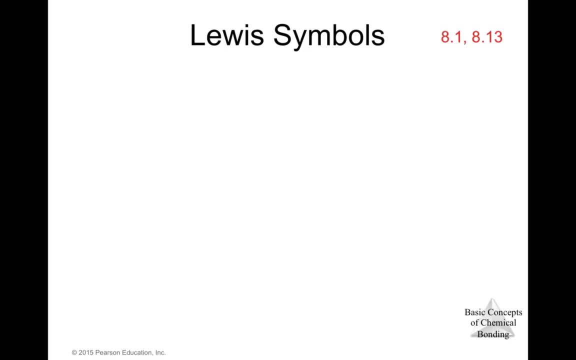 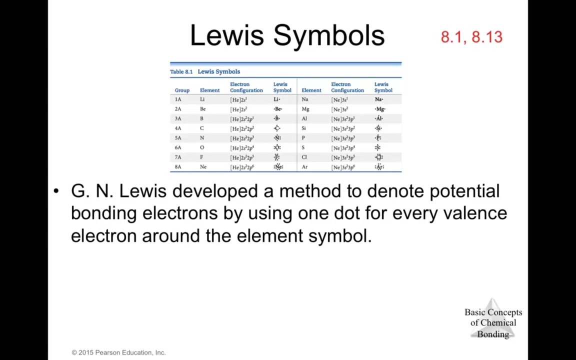 Theð streams of branch crystals are associated to the Integral Conditioning Cycle. The points curves in the cross concentric because they're connected and so items balanced electrons around the element symbol. so, for example, lithium is from family one. that means that lithium has one balanced electrons. so we can write. 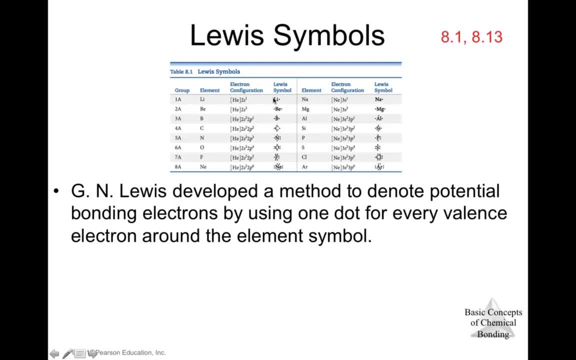 the structure of the Lewis structure or Lewis symbol for lithium as Li and one dot, because lithium is from family one as well as sodium. sodium also is from family one, so we can represent sodium, the structure, Lewis structure as Na and the dot beryllium is from family two, so that's why we can use the symbol of 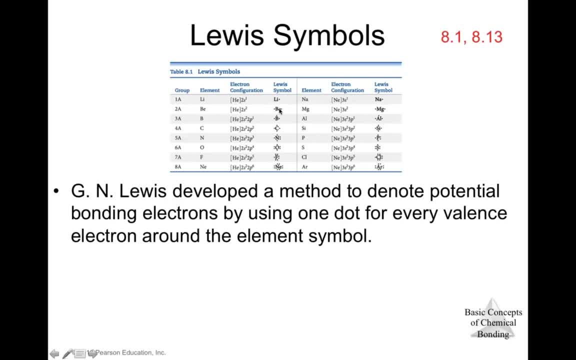 beryllium and two electrons in both sides. we can put two in the left, one in the left and number one right, or one at the top or one the right doesn't matter, but they need to be separate. magnesium also is from family two, so we can have here the magnesium with the two electrons boron family three, so that 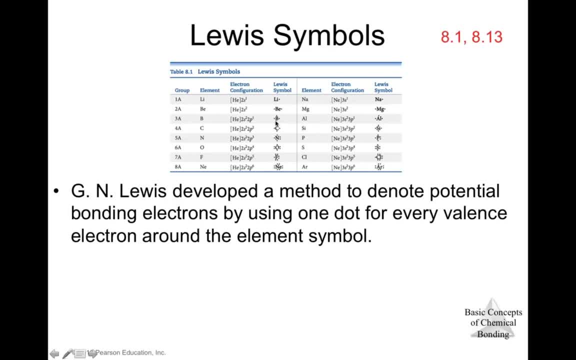 means that it has three balanced electrons. so that's why we write beryllium, the foundation of the company, and that's how we write the earth in the bottom, as a, B, and also we can Draw three dots, each one representing one of those three valence electrons. 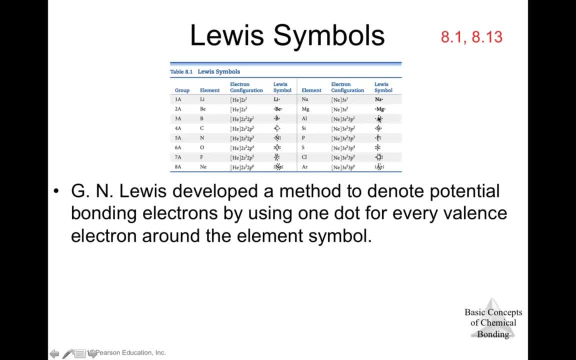 Aluminum as well. family three: we can write the Lewis structure by writing a AL for aluminum and draw three dots Around aluminum. it could be in every of the four position. We can write one here, one in the bottom, one here, one one here when the bottom one the top or any other place. 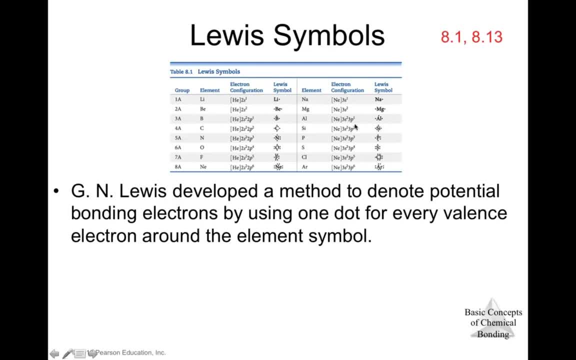 So we have four options to draw each of those electrons For carbon. carbon is family four, so that means that we have four valence electrons. So we need to write those four in each side of the carbon. we have four side: one top, bottom, right and left. So we write one electron in each side, the same. 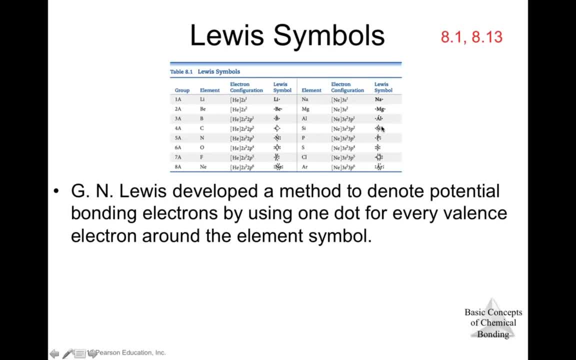 Happened with silicon here, si and the four electrons. now when we get to nitrogen We have five, because nitrogen is a family four- five. so that means that We write four all around the the nitrogen, But we need to pair the fifth electron with any of those four electrons that were alone. okay. 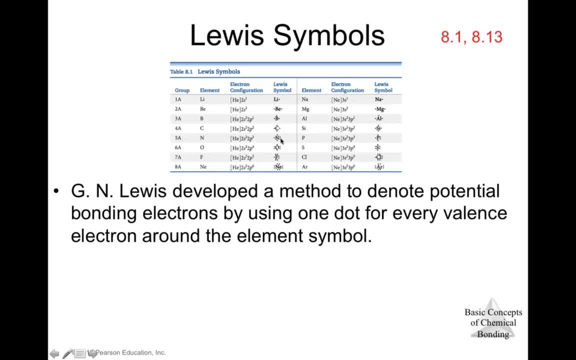 So in this case we can put two electrons here and three Some individual electrons in the other side. We can write the two electrons in the top and one here, one in the bottom, one in the left side, okay? So the important thing is that we're gonna have one pair of electrons and three. 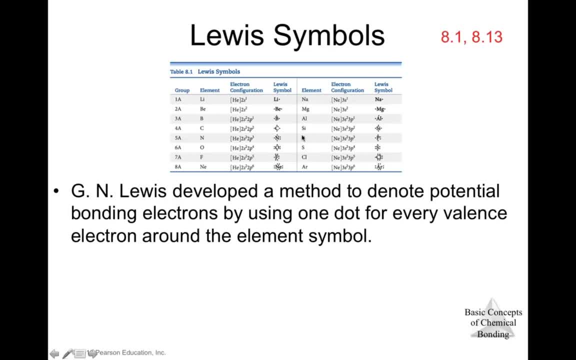 individual electrons around the symbol as well as phosphorous- family five. we have a Long pair here and we have three individual electrons around the phosphorous symbol For oxygen. that is, in family number six. we have in this case two Pair of electrons and also two individual electrons, so we can write two. 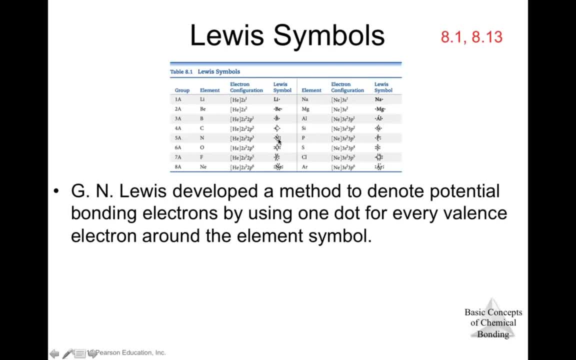 the two pairs on the left, one in the left and the other one the right, and the individual, one in the top or in the Bottom, or we can write one individual on the left, the other one in the right and the two pairs, one top and one of the bottom. so the important thing is that we're gonna have six electron are around the oxygen as well as. 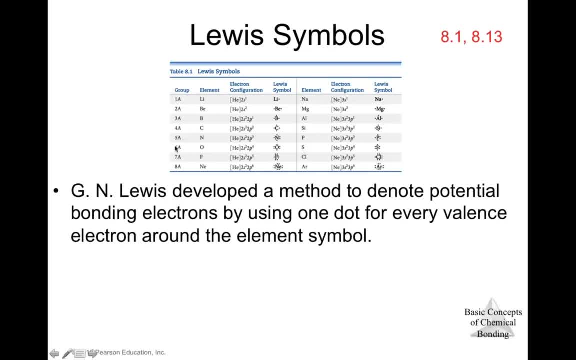 In sulfurs or forces. It's an element from family six, So that means that it has six violence electrons and we can write that around this symbol of sulfur, that is s, we have two pairs of Electrons and two individuals electrons. now we talk about family 7. family 7 means that we have 7 valence electrons and we 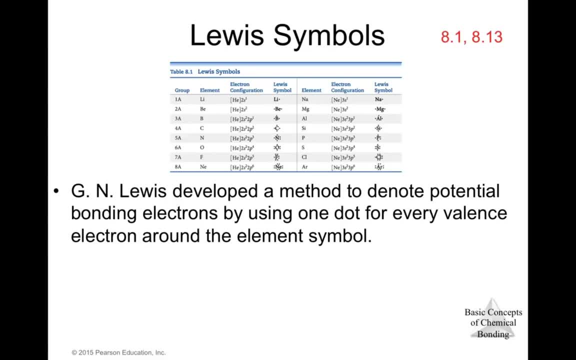 can write those electrons around the symbol, in this case F for fluor, and we're gonna have three pairs of electrons and one individual electron- chlorine, also for family 7. that means that we have seven valence electrons around the chlorine, so we can put three pairs and one single electron, or we 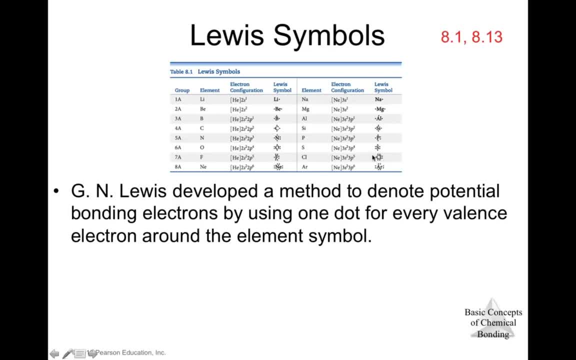 can you put the single electron on the right side and the long pair in the left side, or whatever we have at the? at the end we need to have three pairs of electrons and one individual electrons around the symbol of chlorine and finally, family 8. family 8 are the noble gases and we know that in that case we 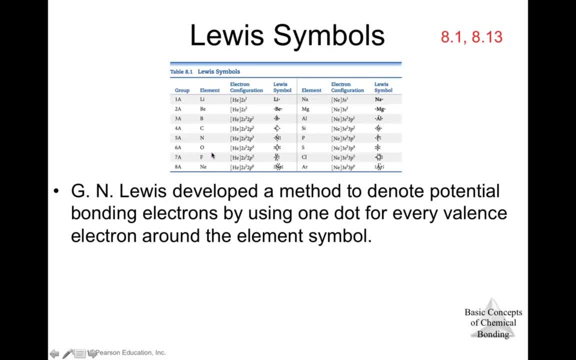 need to write eight electrons around the element, in this case neon. so we have eight electrons. we have four pairs of electrons. argon is also family 8. we can write the symbol structure, Lewis symbol as a are and eight electrons around the argon by using four pairs of. 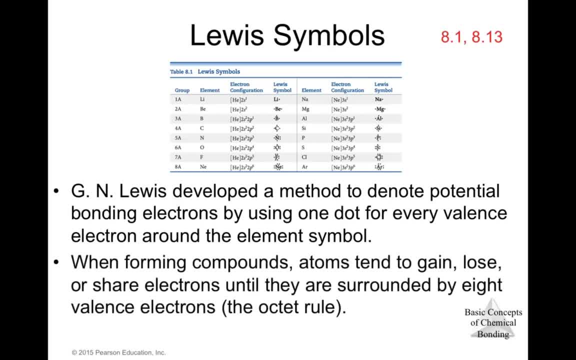 electrons. so when forming compounds, atoms tend to gain, loose or share electrons until they are surrounded by eight valence electrons. that is known as the octet rule. so all the atoms wants to have eight electrons around them and that gives a lot of stability. so that's why we have that the noble. 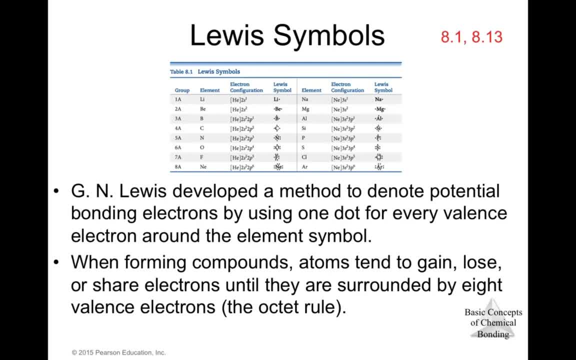 gases. they have eight electrons, so they don't, they are reactive. they don't react with other elements, and other elements are fluorine, for example. they have seven electrons, so they love to gain one more, so in that way they will have the octet rule complete, okay. and for example, sodium. 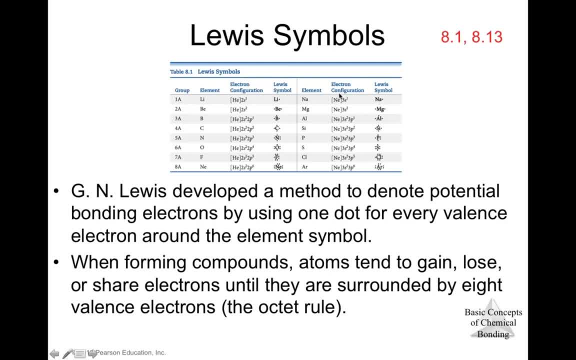 for them is more easy to lose one electron and have the configuration of neon that will complete the octet rule, then gain seven electrons. so for that. that's why in family 1, as we know, all the elements and atoms for family 1, they has a positive one charge as an ion, because for them it's really easy to 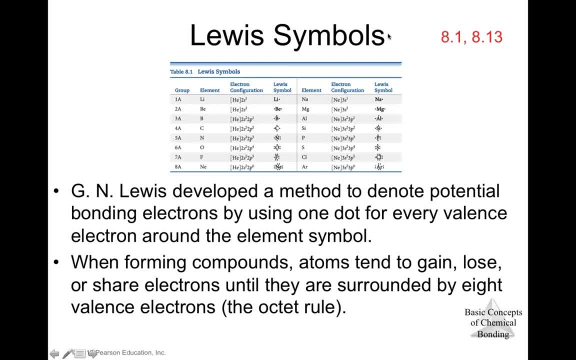 remove that electron so in that way they can have the configuration of neon. that is a noble gas, and all the noble gas has the octet. so that's why it is easy for them to remove one electron: magnesium and beryllium family 2. for them is really easy to remove those two electrons. 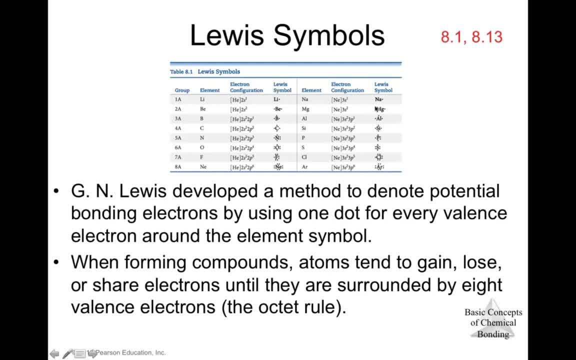 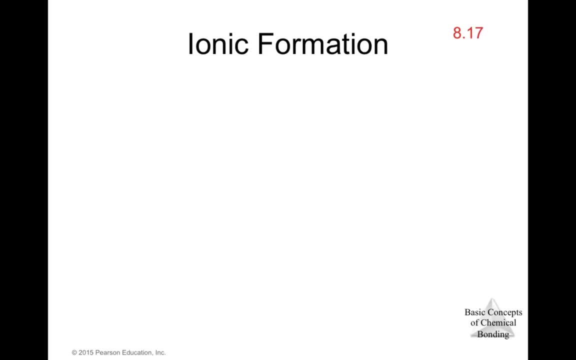 that's why family 2 always gonna be plus 2, because when they do that now, they have the configuration of a noble gas. so let's talk now about the ionic formation. ionic substances generally resolve from interaction of metals that are in the left side of the periodic table with non metals that we can find them at the 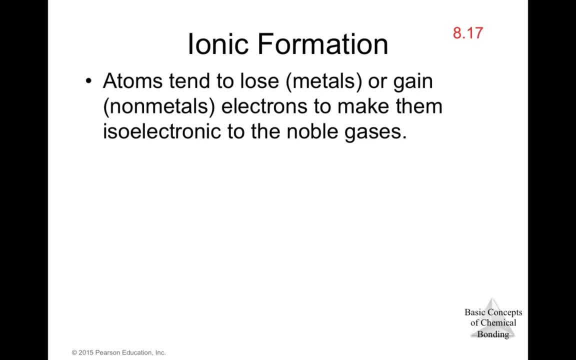 right side. okay, so most of the time the metals are the ones that like to lose electrons and the nonmetals are the ones that gain electrons and in that way, basically, they can eventually create that novel configuration or configuration of novel gas. for example, we have sodium here and we have 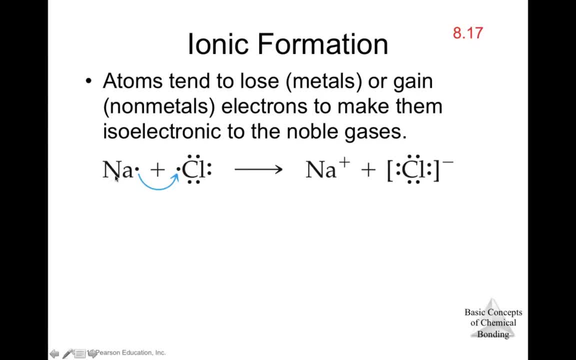 chlorine. these are the new structure for sodium and for chlorine. sodium is for family one, so that's why we write na and one electron. chlorine is from family seven, so that's why we write three pairs of electrons and one single electron and, as we mentioned, in this case we have a metal and we have a non-metal, so the metals. 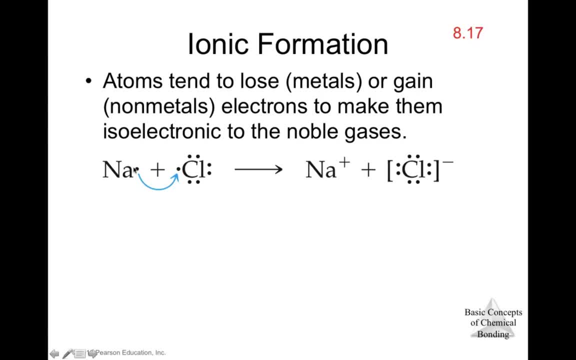 tend to lose that electron, so they release that electron. and chlorine, that is from family seven. they love to gain electrons. okay, so in that way now we are as when we release that electron. now the sodium has a positive one charge. it was neutral before, but because we remove one negative particle, 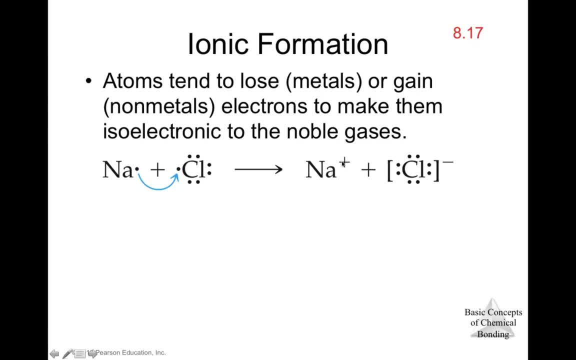 now this, the sodium percent is going to have a positive charge like a time, and chlorine will receive one extra electron. here was neutral, but when you receive that negative particle particle, now you have eight electron. you complete here your octet. so you complete the octet rule and you're going to be negative one. 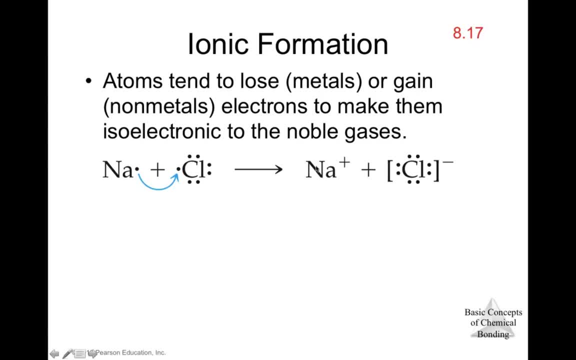 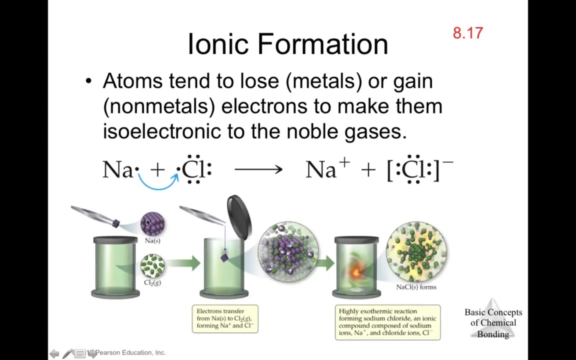 because you gain that electron, sodium, and also because they lose that electron, they will gain that electronic configuration from the novel gases, and this that's why we can create those ions and we can have that ionic compound as sodium chloride. so here we have, for example, the sodium. 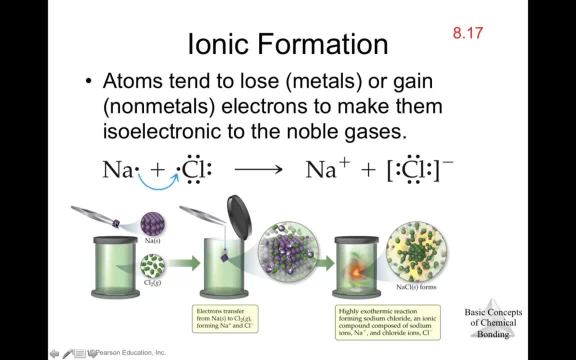 as a solid and we have the gases, chlorine. we combine them in this chamber and at this point they start to the sodium, start to release those electrons are trans, being transferred from the sodium to the chlorine gas and because they transfer, that they are losing those electrons, we start to produce the 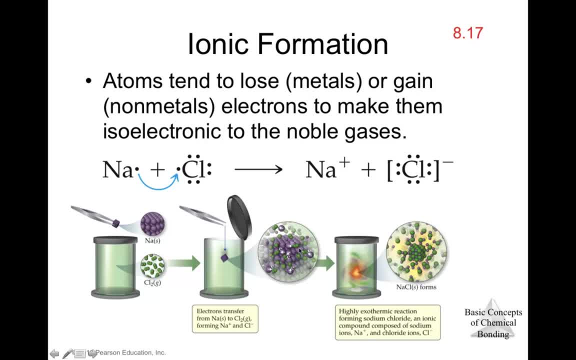 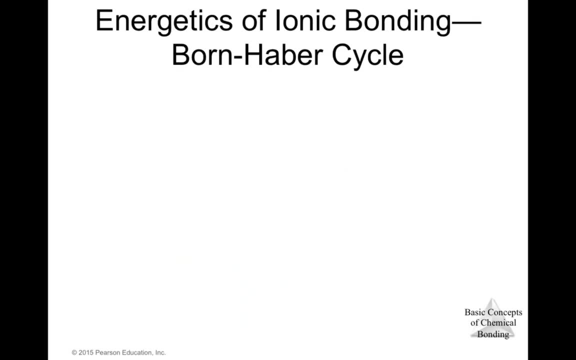 sodium ions and also as well, when chlorine received, those electrons start to produce the chlorine ion and eventually they will form sodium chloride and this, basically, is known as an exothermic reaction. so let's talk about the energetics of ionic bonding, specifically the Born-Havard cycle. many factors affect the energy. 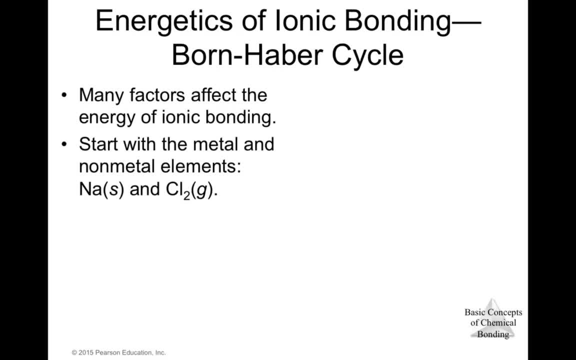 of ionic compounds, or ionic bonding, start with the metal and the non-metal element. as we saw before, we have the sodium as a solid and the chlorine as a gas. then we need to make them transくain like gaseous atoms. okay, so the sodium gas will produce, the sodium solid will turn. 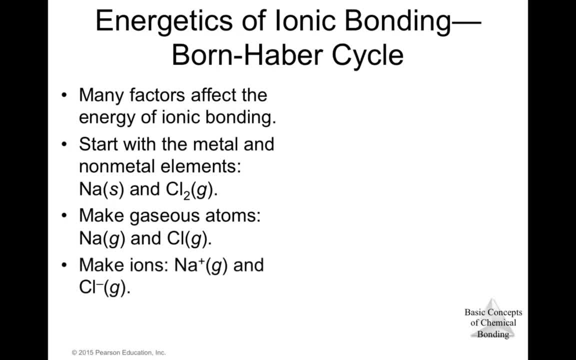 in gas, and then we need to create those ions and then those ions will combine to produce the sodium chloride, the molecule of sodium chlorine, our ionic compound. so this is, uh, the the Born-Havard cycle for this type of reaction, where we have initially the sodium as solid and chloride metal and as a gas. 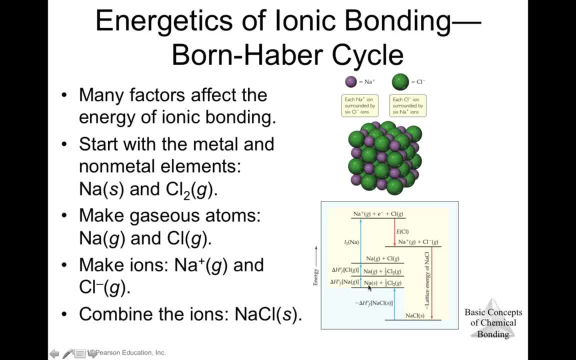 is a gas. we transform this gas to this solid, to the gas, and at this point we have the ions produced. this process, all this process, absorb energy, so that's why the energy is increasing. but then, when you start to combine the ions, you will produce the sodium chloride and this. 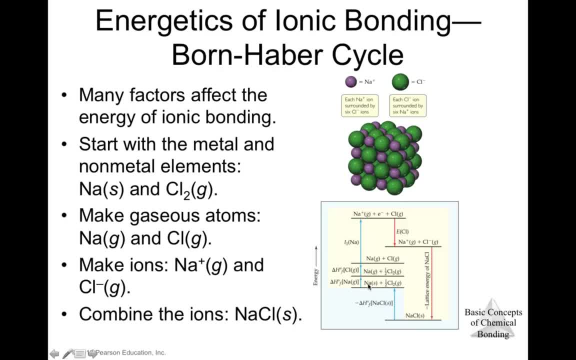 sodium chloride has a lower energy than the initial reactants, so that means that this process, the whole process, is an exothermic process. you start at this point in energy and you finish at this point in energy and the total energy of this process. for this, the production of sodium- 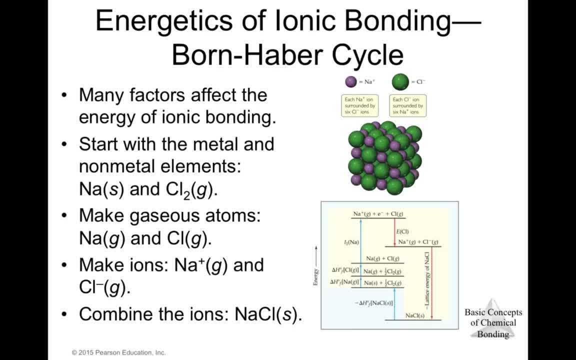 chloride is seven hundred and eighty eight kilojoules, and this is also associated to the lattice energy for sodium chloride. okay, so sodium chloride, basically, this process to produce will will release a total of 788 kilojoules per mole, and this is also associated to the lattice energy, because 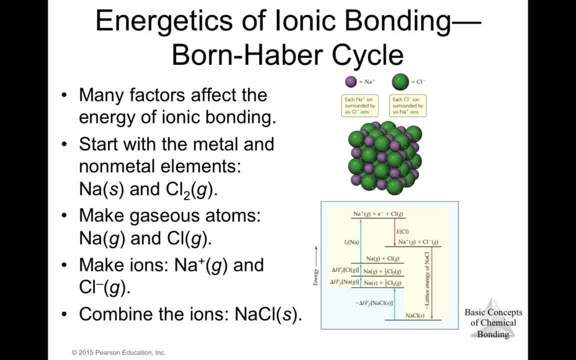 an exothermic. if you're talking about the energy that is released, you will see that it's negative- 788 kilojoules. but the positive of this value, that is, 788 kilojoules, is the lattice energy, the energy that you will need to add to the 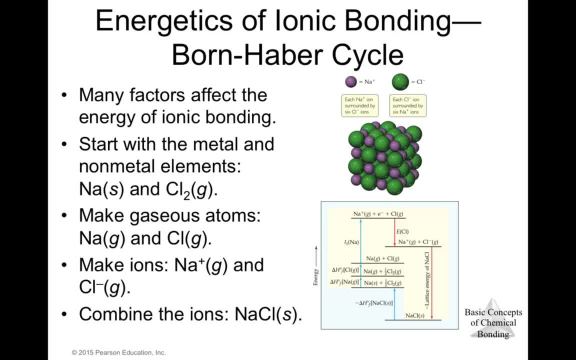 sodium chloride to separate those ions. okay, so deformation will release 788 kilojoules. that's why, as when it released, you're going to have a negative, negative value. but if you want to separate those ions, if you start, for example, with sodium chloride and you want 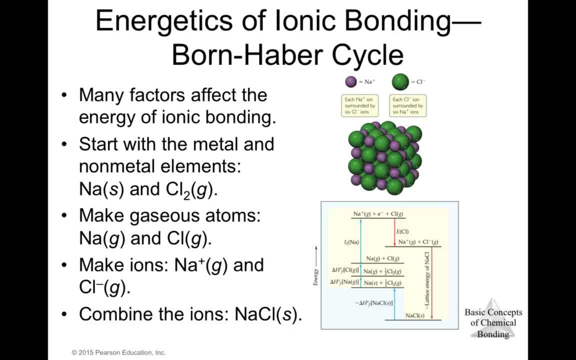 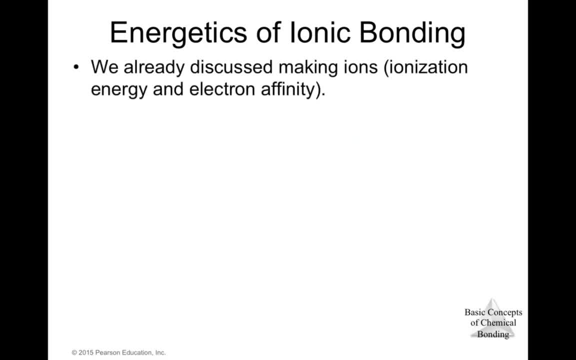 something like chlorethrane and you want something like tranexamine and you start separate those ions. you will need to add 788 kilojoules to separate those ions. so we already discussed that: making ions, ionization energies and electronic affinity. remember that the ionization energy is how easy is to create an ion. 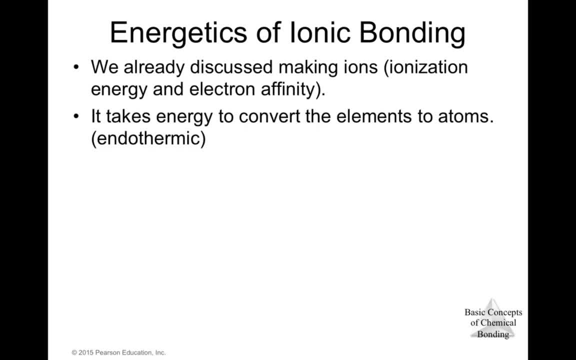 and in this case, how is to release the electrons? so that's why the cations has basically those ionization energy, while the nonmetals you talk about the electron affinity, because they will like to gain those electrons. it takes energy to convert the elements to atoms and then the thermic process. it takes energy. 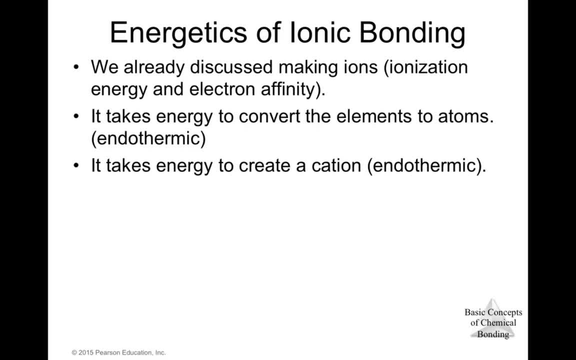 to create a cation and the thermic process, as we saw in the cycle in the past, slide. but energy is released by making the anion and also the formation of the solid release a huge amount of energy. and it is released by making the anion and also the formation of the solid release a huge amount of energy. 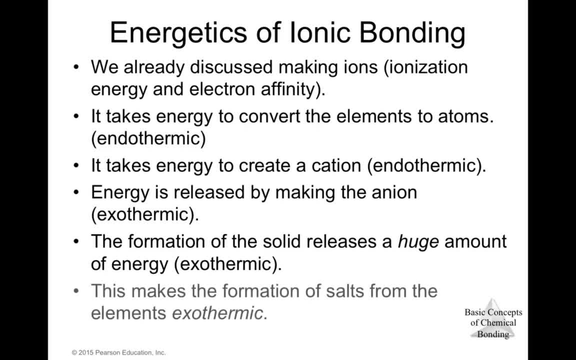 being an exothermic also reaction. so this make the deformation of the salts from the elements is exothermic, as we saw before. we saw that the energy of the sodium chloride is lower as the energy of the reactants. so that's why this process to produce sodium chloride is an exothermic kind of reaction. 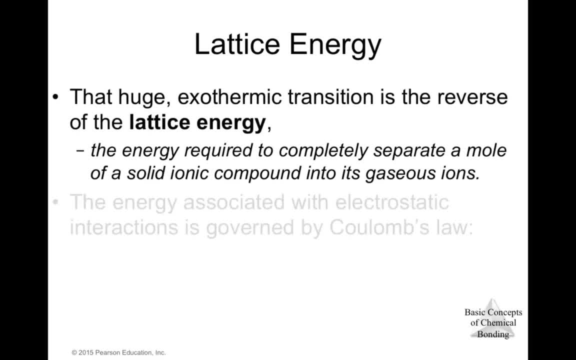 the lattice energy, as I mentioned before. in this case that huge exothermic transition is reversed. that is the reverse of the lattice energy, the energy required to completely separate a mole of solid ionic compound into its gaseous ions. so we saw how to, from the gaseous ions, create that solid, and that process was minus seven hundred and 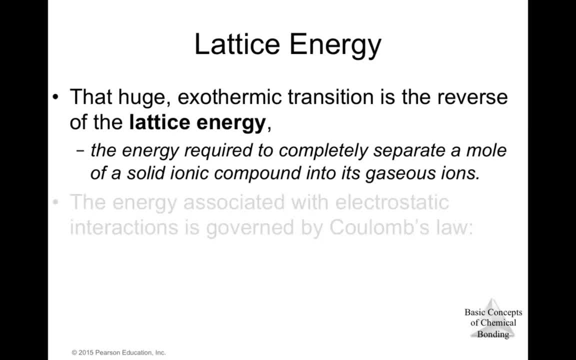 eighty eight kilojoules. but now if you have the solid ionic compound and you want to return there to gaseous ions, you need to add 788 kilojoules per mole. for the sodium chloride, The energy associated with the electrostatic interaction is governed by the Columbus law. 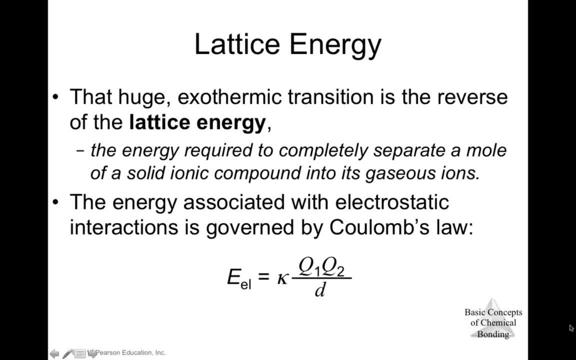 That electrostatic interaction here is equal to kappa times Q1 and Q2 divided by D. In this equation, Q1 and Q2 are the charges under particles in Columbus With their sign n. D is the distance between their centers in meters. 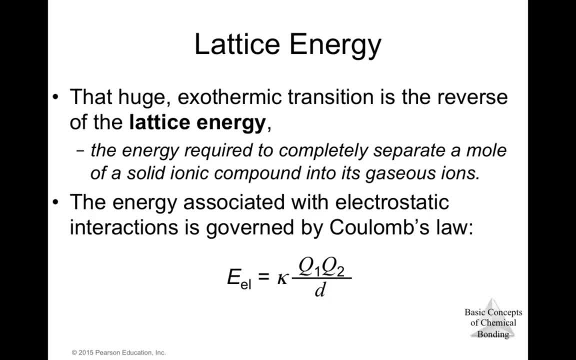 And kappa is a constant. So basically, this equation indicates that the attractive interaction between two oppositely charged ions increases as the magnitude of their charges increase and as the distance between their centers increase. So that is the equation we hear- decreases. thus, for a given arrangement of ions, the lattice energy increases as 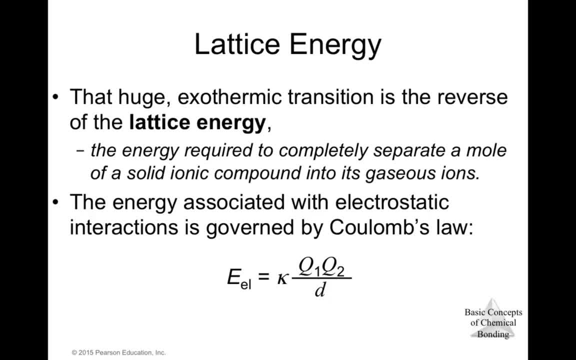 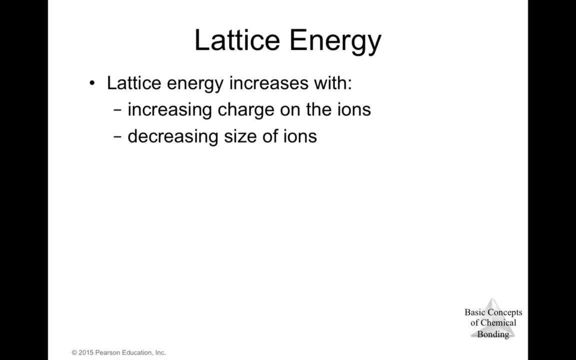 the charges on the ions increases and, as they're ready, decrease. so that's why it is important to understand this Columbus. this Columbus basically gave us that relationship between the charges and the distance that they're really important for that lattice energy. you, so the lattice energy increases with increasing charge on the ions and 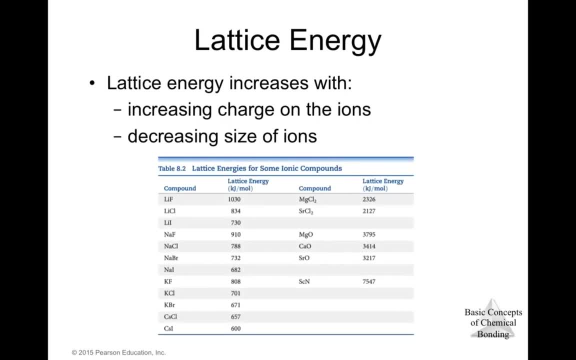 decreases size of ions. so here we have the lattice energy as we can see here, lithium: when you combine lithium with fluorine, chlorine, iodine, fluorine is smaller than chlorine, chlorine is more than iodine. so I guess you guys can you see that any lattice energy will increase when that size of the ion is. 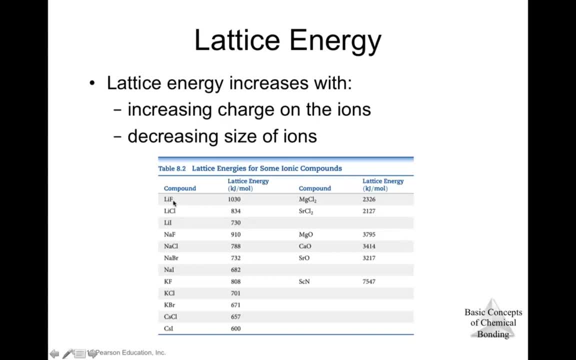 small. the lithium is constant, so it's not making any difference. any difference here. the one that is changing is the anion, as as you increase the size of that anion, the energy will decrease. so that's why the energy will increase when you will decrease the size and also increase in charge on the ions, as we can see here, we 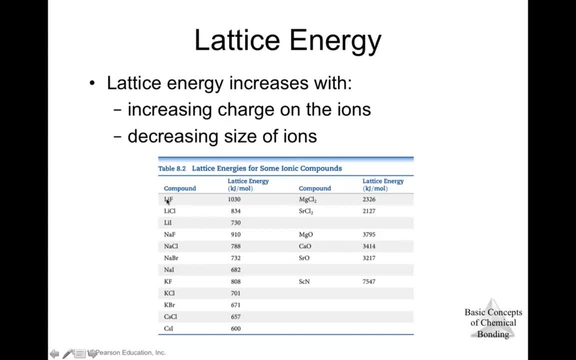 have lithium, we have magnesium. lithium has a positive 1, magnesium a positive 2. so that means that we are increasing that charge and what happened to the lattice energy also increase. so the lattice energy will increase with an increasing charge of the ions and by decreasing the size of the ions. 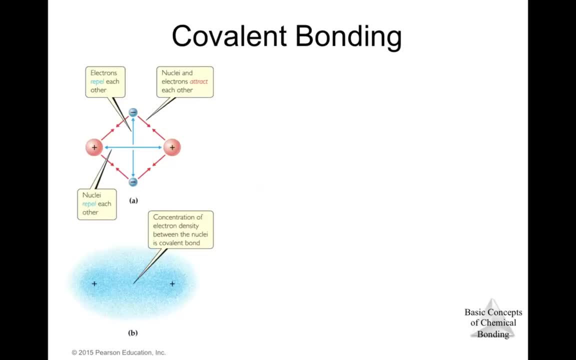 so let's talk now about the covalent bonds. in covalent bonds, atoms share electrons. okay, in ionic they transfer from the metals to the nonmetals. it's a transfer of the electrons. that's why you create ions and that's why it's called an ionic bond here. in the covalent 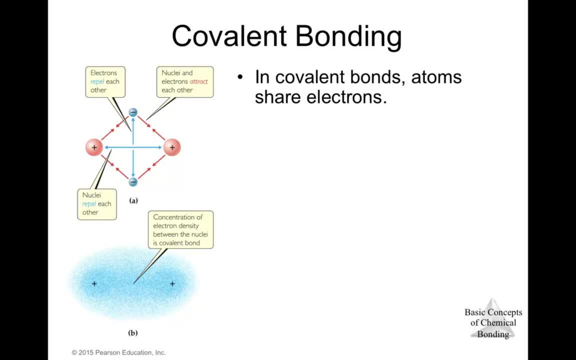 bonding. the electrons are shared between those atoms. there are several electrostatic interaction in these bonds, attractions between the electrons and the nuclei. remember that the electrons is a positive charge because in the nuclei we have a positive charge, because we have there the protons. so that's why you 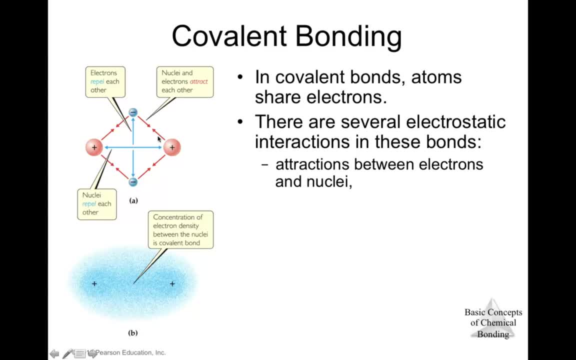 have an attraction between the nuclei and the electrons also you will have repulsion between the electrons- this and this electrons is gonna have some kind of repulsion- and also between the nuclei, because also they have a highly concentration of positive charge here and also here there's gonna be a 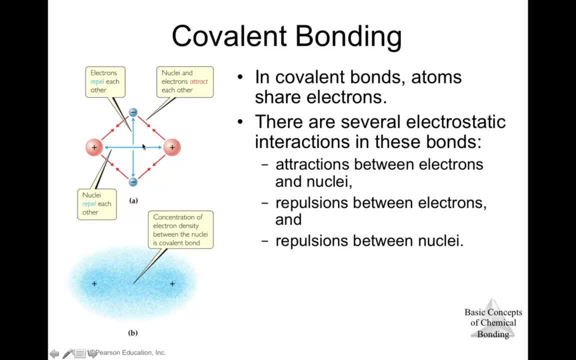 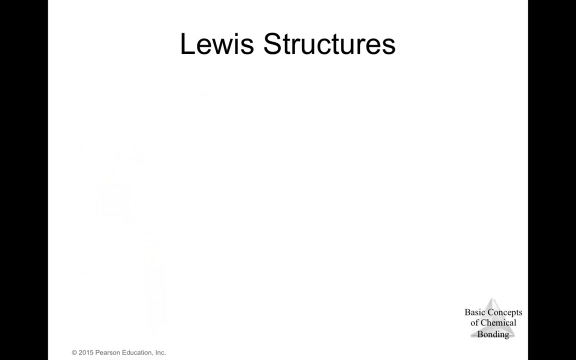 tendency also to separate a little bit those nuclei due to the repulsion for the high concentration of positive charges. for a bond to form, the attraction must be greater than the repulsion. for covalent bond to form, the attraction must be greater than the repulsion. so let's talk about the Lewis. 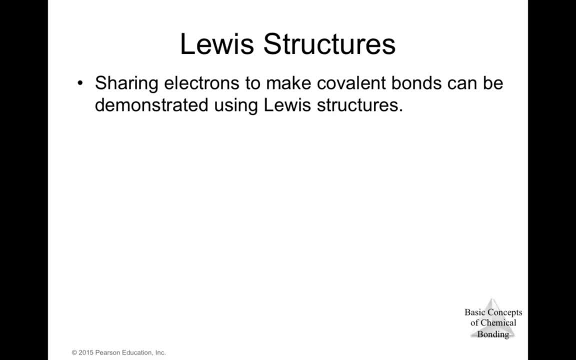 structure and see how that this can help us with the covalent bond sharing electrons. to make covalent bonds can be demonstrated by using the Lewis structures. we start by trying to give each atom the same number of electron as the nearest noble gas by sharing electron. remember that he wants. 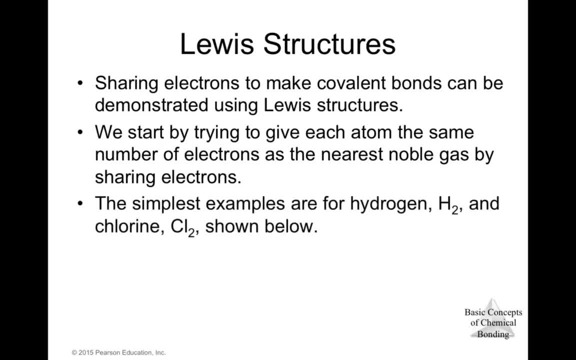 to complete that opted rule. the simplest examples are for hydrogen h2 and chlorine cl2 that we're going to see here in a moment. in the case of hydrogen, we have that hydrogen is from one, so that means that each hydrogen is going to give one electrons. so here this. 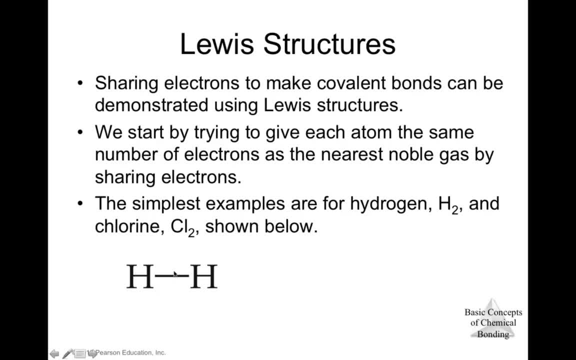 bond has the two electrons, one from this hydrogen and the other one from this hydrogen, so each bond always are going to have two electrons. in the case of chlorine, chlorine is from family seven. okay, remember that chlorine is from family seven. so we have here two electrons in this bond and here we have 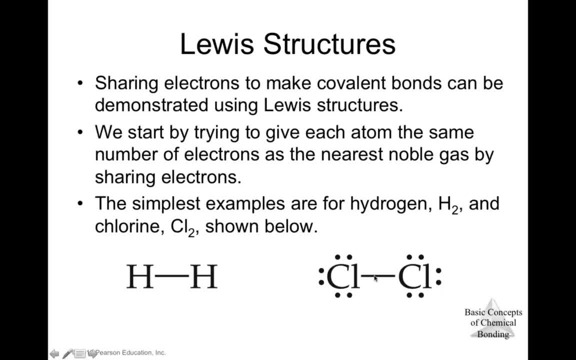 two, four, six plus one of this is going to be seven and two, four, six plus one of this. remember, we're going to have two here, one from here and one for here. we have, we still have the seven, but now, because they are sharing this, two electrons. that means, as those two electrons are from this chlorine and 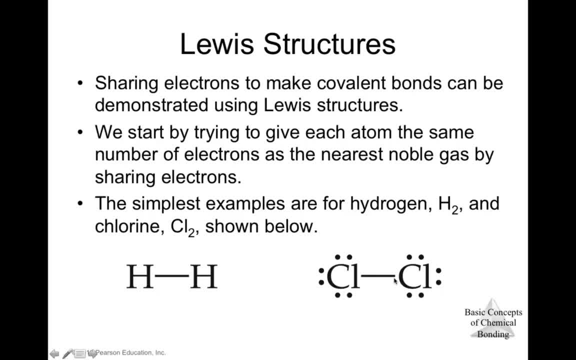 also from this chlorine. so now, because we are sharing this two electrons, we have two electrons here we have two, four, six and eight. so here we have the octet rule complete, as well as in this chlorine, because we have two, four, six, and this two that has been sharing by the two atoms of. 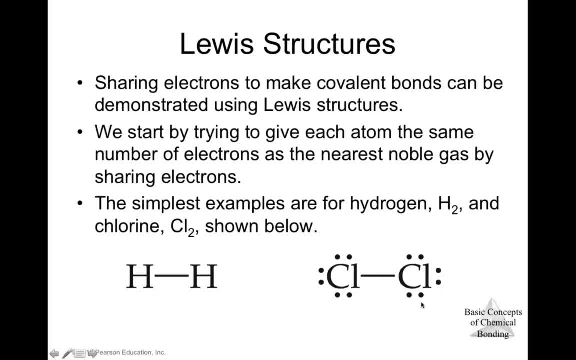 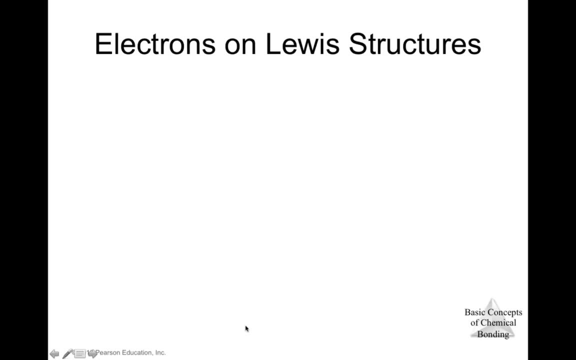 chlorine complete the octet rule for this chlorine. okay, so now we have the octet complete here because we have eight electrons around this chlorine, And we also have eight electrons around this chlorine because we are sharing two electrons. So electrons on the Lewis structure, long pairs Electrons located and only one atom in a Lewis structure. 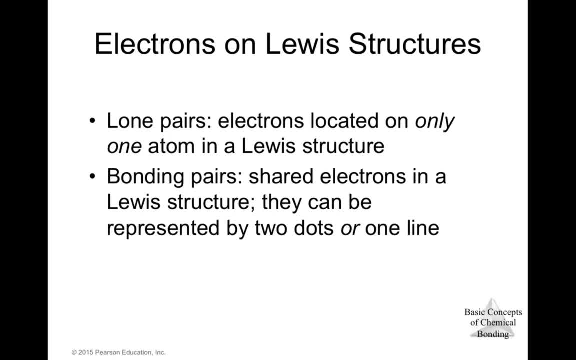 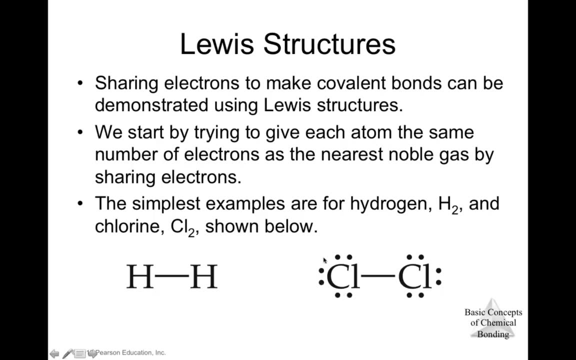 So those are the long pairs and the bonding pairs, the share electrons. in a Lewis structure They can be represented by dots or one line. So, as we saw here, let's go pretty fast, Fast back. here We have the. these are the long pairs electrons, Okay, and these are the shared electrons. So these are the long pair electrons and the shared electrons. 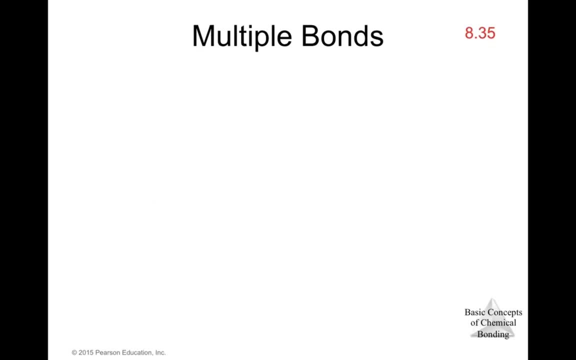 In many molecules, atoms attain complete octets by sharing more than one pair of electrons. In this case we have that some atoms share only one pair of electron and these bonds are called single bonds. But when two electrons pairs are shared by two atoms, two lines are draw in the Lewis structure and this will be a double bond. and 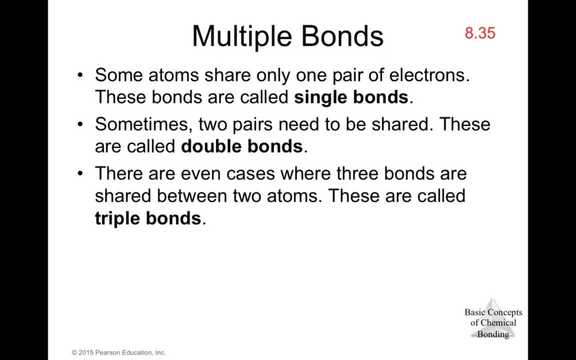 sometimes, instead of sharing just two pairs of electrons, we're gonna have Atoms that need to share three pairs of electrons, so in that way they can complete the Octet rule, and this is known as a triple bond between those two atoms. So here we have an example. 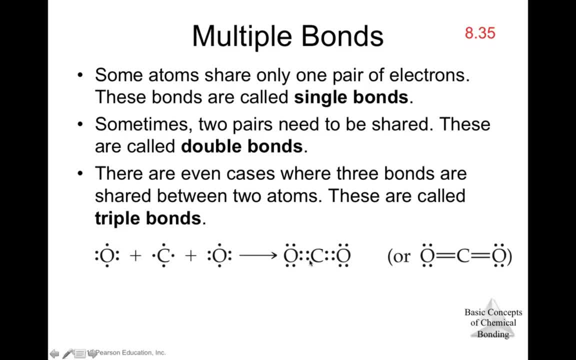 of Carbon dioxide, and between this oxygen and this carbon we're sharing two pairs of electron, as well as from this carbon And this oxygen. we can see here that we have two pairs of electron- has been shared between these two atoms. Once again, this arch has been shared by these two atoms. 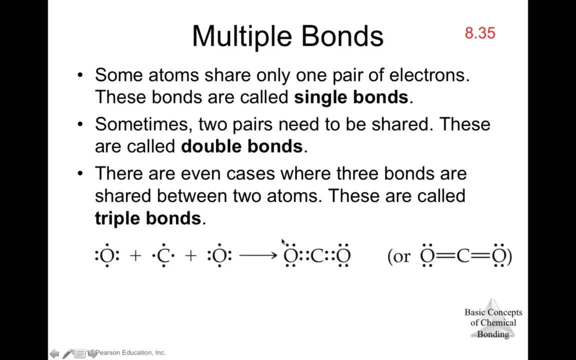 so we have two, four, six and eight electrons around this carbon. and this carbon has Eight electrons. here I mean four electrons shared in this and this side by this oxygen and four here shared with this oxygen. So at a total of eight electrons around the carbon, even though there has this arch. 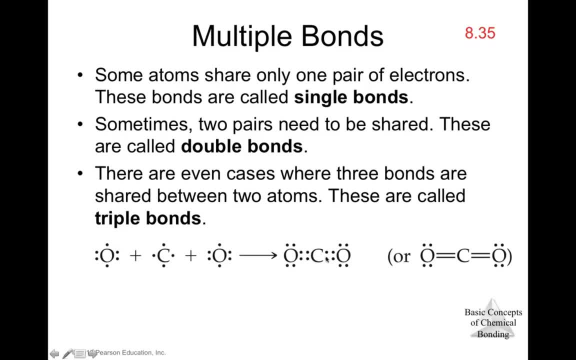 Is it sure you're. the carbon is sharing those electrons now here, but they are around the carbon, So we have eight electrons and that complete the Arctic rule for this carbon as well. for this oxygen We have two long pairs, But also we have four electron that is being sharing by the two. 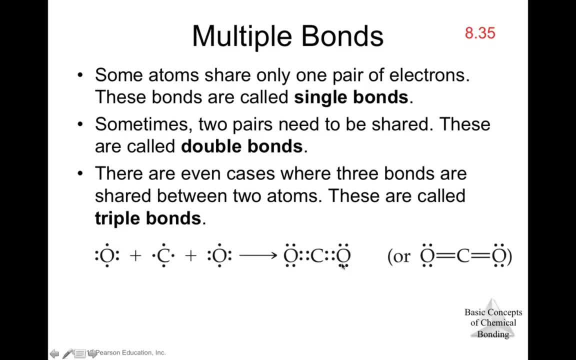 Atoms. so in that way this oxygen also has the eight Octet rule. so we can represent this by drawing the two dots between the two pairs dot between the two carbon or Also by two lines. so that means that each line Represent two electrons. so here we are sharing four electrons and there's this side for electrons. 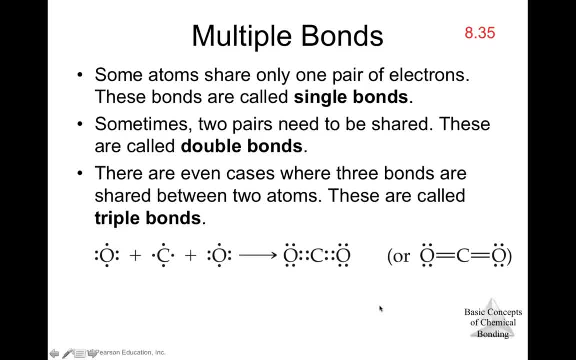 So this is an example of double electron-Rocker bonds and also we can have, for example, in nitrogen they the day. between those two atoms they are sharing three pairs of electrons, so we have basically what is known as a triple bond. so here we have a total of six electron two. 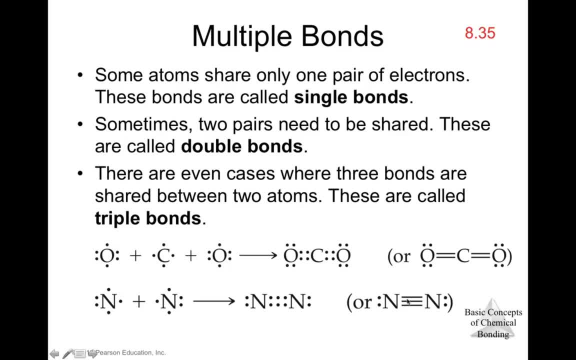 electrons for each bond. so we have six electrons here and two here. around this nitrogen we have eight electrons. we have six electrons here, a pair here, so that means eight. so around this nitrogen we have eight electrons. so we complete that there the octet rules for those two atoms. 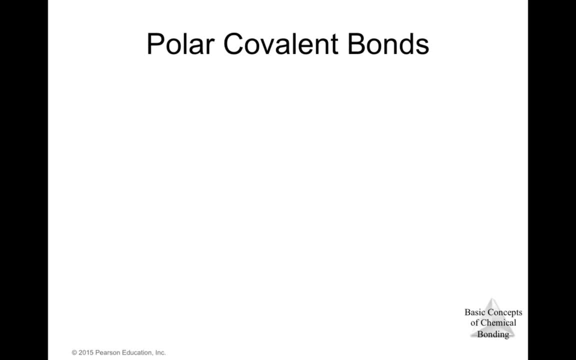 so now let's talk about the polar covalent bonds. when two identical atoms bond, as chlorine or hydrogen, the electron pairs must be shared equally, so those electrons are in the middle between those two elements. so that is known as a non polar covalent bond, but we have also polar covalent bonds. in this way, the 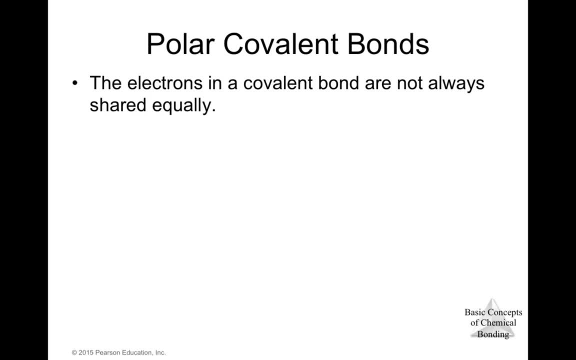 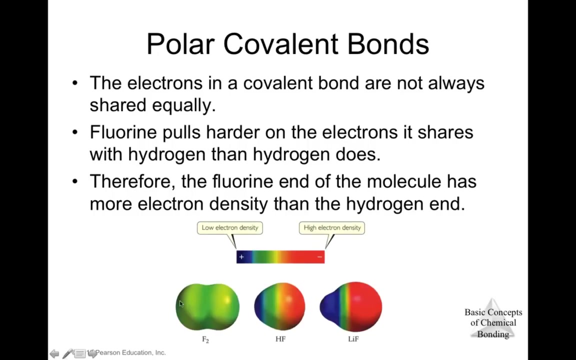 electrons is in a covalent bond are not always shared equally. chlorine pulls harder on the electrons it shares with hydrogen than hydrogen does. therefore, the fluorine end of the molecule has more electron density than the hydrogen, and so here we have, for example, this, our electron density. 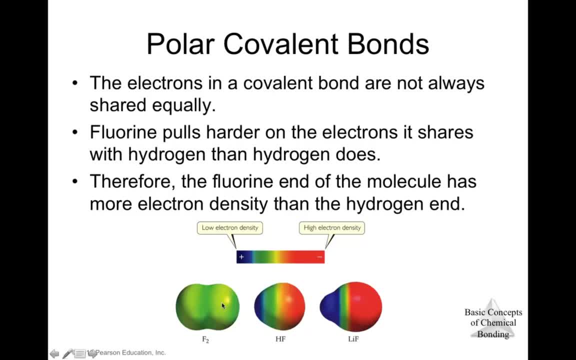 between in a molecule of fluorine, both of them has, basically they pull the the same with this, with the same force. okay, those electrons. so those electrons are basically in the middle of the two molecules. they are sharing those two electrons and they are in the middle now when we put hydrogen and fluorine. 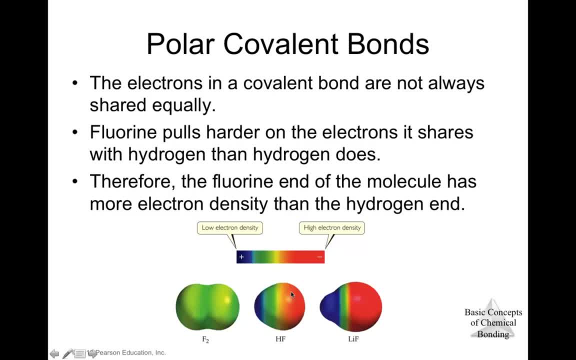 fluorine pulls more those electrons close to the fluorine. so that's why you can see here here a high electric density as compared to the end of the hydrogen. so because fluorine can pull more those electrons, you are creating this polarity in this bond. this side is more negative, this side is more positive. 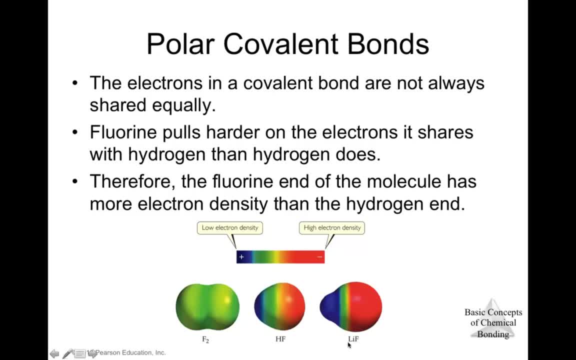 and if we you see lithium and fluorine, there's an ionic compound. we can see here that we have a really positive over here and we have here a high density of electrons with a negative charge in this side in a cut in an ionic compound. okay, 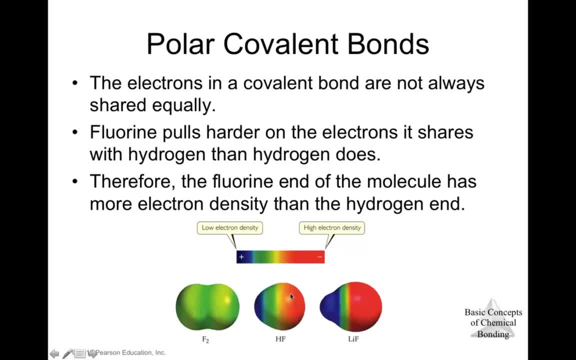 but this one that is covalent. we can see also that we have a higher electron density in this side, because fluorine is in the middle of the two molecules. so that's why you can see here that we are pulling more those electrons that still are sharing with the hydrogen. okay, it's. 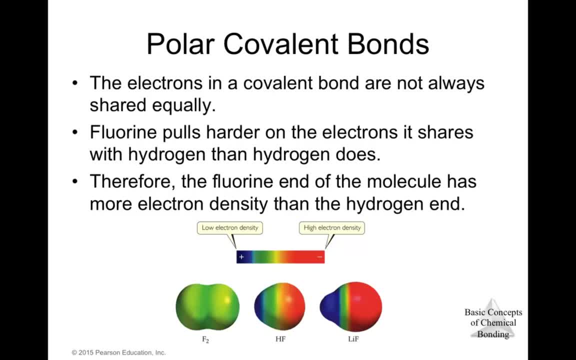 not like they are taking the weight, those hydrogen, those electron from hydrogen. no, they are still sharing those electrons with hydrogen, but they pulled those electrons a little bit more than the hydrogen. so that's why you create that polarity in those covalent bond. so you're gonna have also pull out, well not? 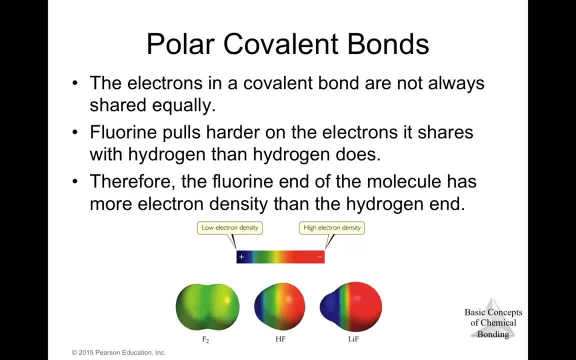 always. but you can have non polar covalent bonds and polar covalent bonds, but you will never have a polar ionic bond, because when you have an ion you're not sharing nothing, you're transferring the whole electrons from the metal to the metal. so when you're talking about polar or nonpolar is when you're talking. 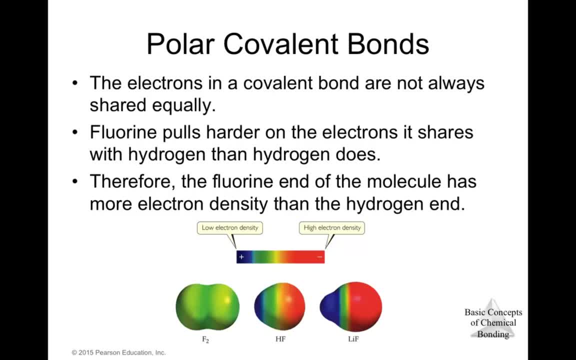 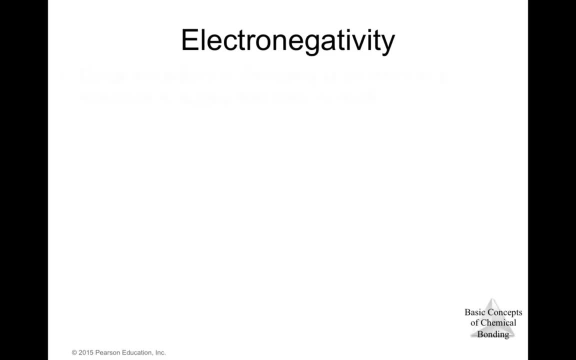 about the covalent bonds. we use a quantity called electron negativity to estimate whether a given bond is nonpolar covalent, a polar covalent or an ionic, and that's your negativity. is defined as the ability of an atom in the molecule to attract. 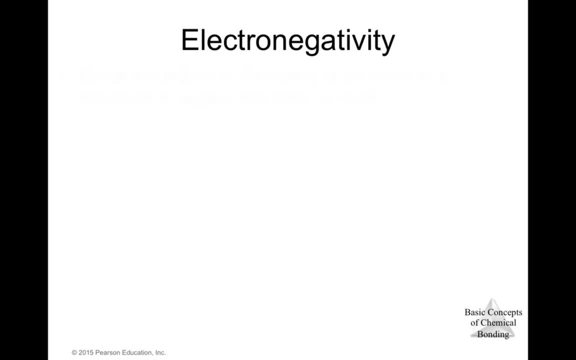 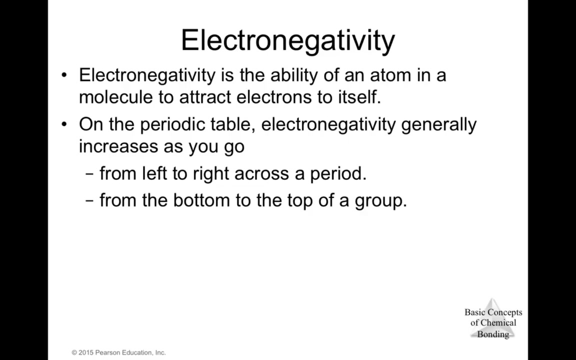 electrons to itself, the greater and atoms electronegativity, the greater its ability to attract electrons to itself. so, as mentioned, is the ability to attract those electrons and in the periodic table there is also a trend: Electronegativity generally increases as you go from the left to the right across a period. 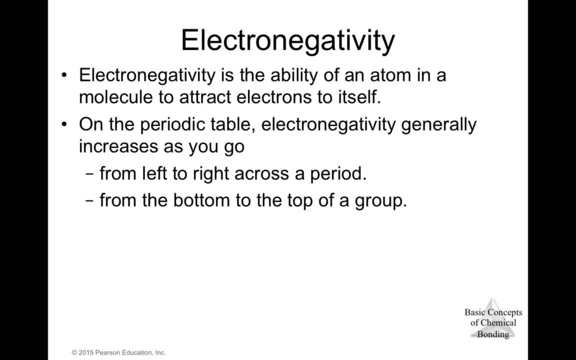 and when you go from the bottom to the top in a group. So that means that the highest electronegativity is found in the fluorine. That's the atom that is in the right side and is in the top side of the group. So this fluorine is going to have always the highest electronegativity. that 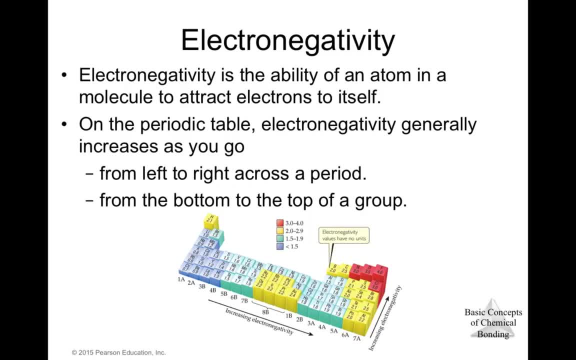 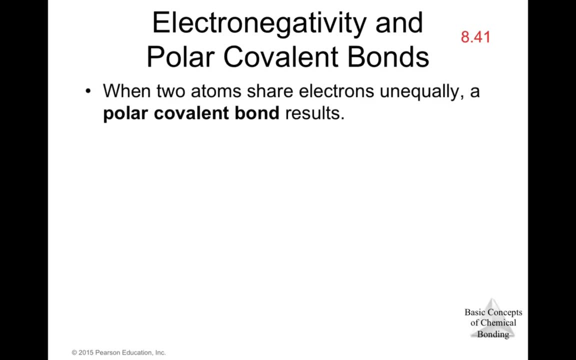 is established as 4.0.. That's the electronegativity of fluorine, the one that has the highest electronegativity. So electronegativity and polar covalent bonds: When two atoms share electrons unequally, a polar covalent bond results. 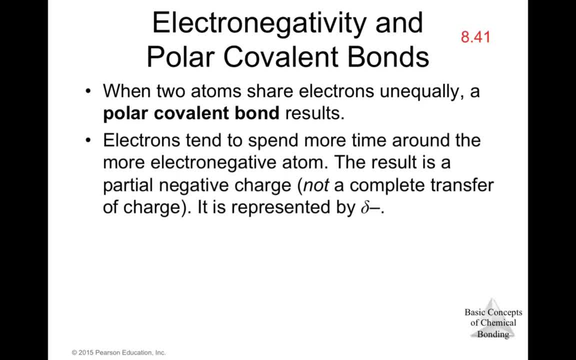 Electrons tend to spend more time around the more electronegativity atoms. The result is partial negative charge and it's represented by this symbol that is called delta, Delta, negative. Okay, so that's when you create that polarity in the bond You're going to identify which. 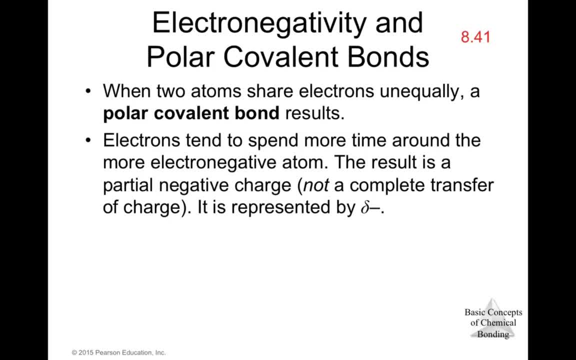 which end is negative and which then is positive, by using the delta minus or delta plus. the other atom or the other n is going to be the delta plus, that is the more positive n. so here we know that fluorine is going to pull all those electrons, both of them one, from hydrogen. 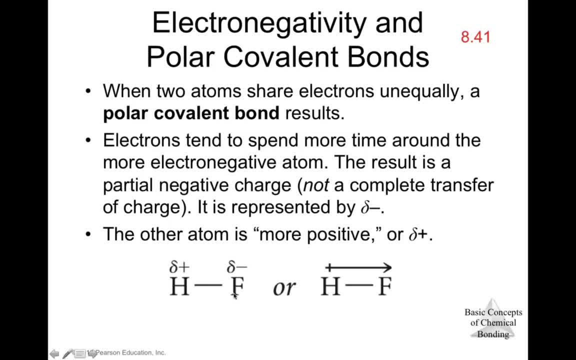 one from fluorine. they're going to pull them close to the more to the fluorine, so we're going to represent this as delta minus, and the hydrogen that is is feeling that it doesn't have those electrons close to it, so you're going to have a partial positive charge, so it's represented by the. 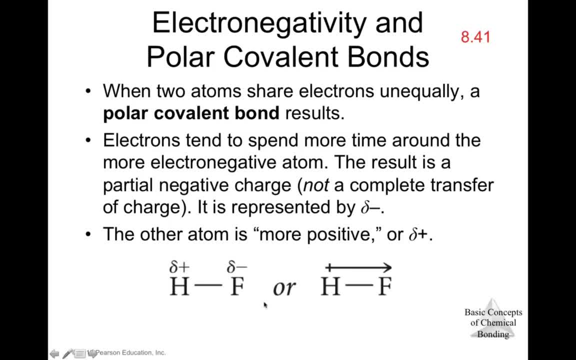 delta positive, partial positive, partial negative. also, another way to represent it is by using an arrow: okay, and the head of the arrow is going to be in the more high density electron. okay, or the delta minus, and the cross of the arrow is going to be in the more positive end, or the delta positive. 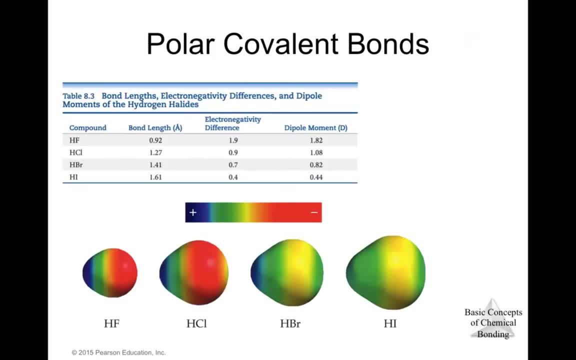 so here we have the polar covalent bonds. again we have a table and we can see here the electronegativity difference between hydrogen and fluorine, hydrogen and chlorine, hydrogen, bromine hydrogen and iodine and also the bond length and we can see that the hf has a higher uh dipole. 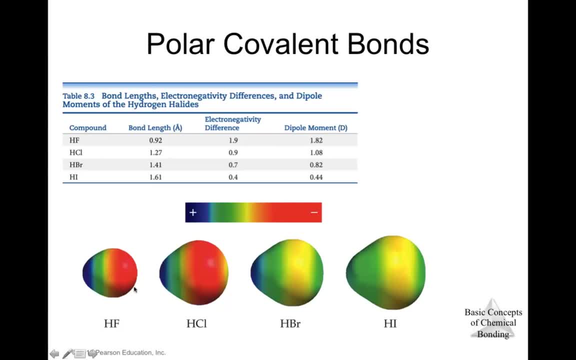 moment. that means that we have a partial negative or very high partial negative density here and a partial positive. okay, and this has a big dipole moment because, one, the electronegativity difference between these two and also because of the bond length that is really small. so hcl. 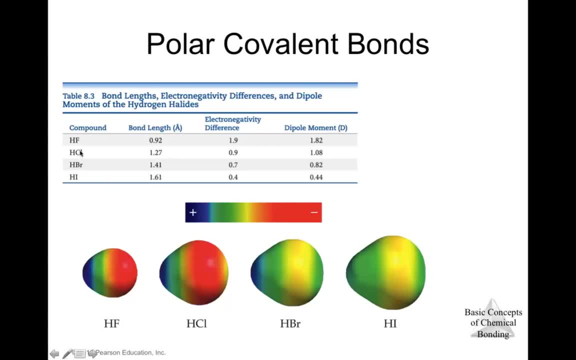 here have a larger anion. the bond length is a little bit longer, okay, and the difference in electronegativity is 0.9. the dipole moment is 1.08 is still being considered a polar covalent bond. hbr also has a larger bond length, electronegativity difference of 0.7. 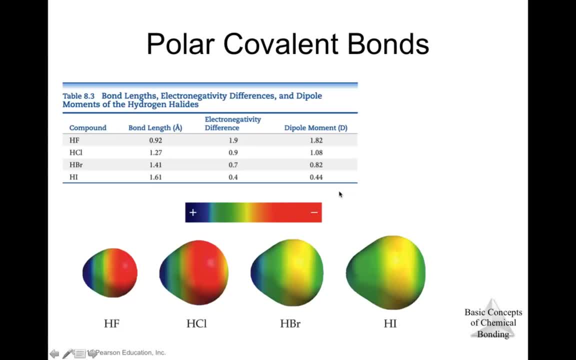 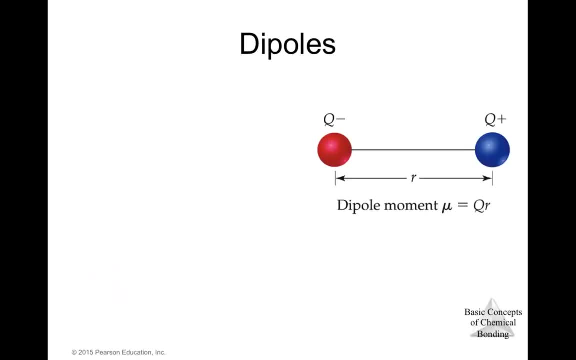 dipole moment of 0.82, also considered as a polar covalent bond, as well as the h? i. clarity helps determine many properties we observe at the macroscopic level in the laboratory and in everyday life. polar molecules align themselves with respect to one another with the negative. 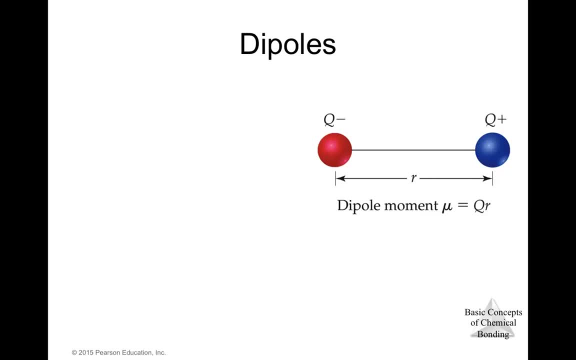 end of one molecule and the positive end of another attracting each other. polar molecules are likewise attracted to ions. the negative end of a polar molecule is attracted to a positive ion and the positive end is attracted to a negative ion. these interactions account for many properties of liquid, solids and solutions. how can we quantify the polarity of a molecule whenever? 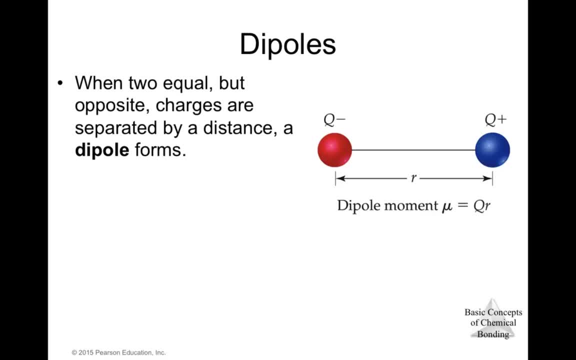 two electrical charges of equal magnitude but opposed sign are separate by the distance, a dipole is established. the quantitative measure of the magnitude of a dipole is called the dipole moment, represented by the greek letter mu. if two equal and opposite charge, q positive and q negative, 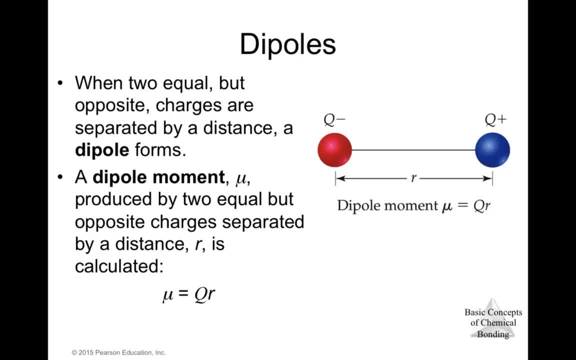 are separated by this. on r, the magnitude of the dipole moment is the product of q times r. so this, basically, is the expression of the dipole moment, and the dipole moment will increase as the magnitude of the charges increase and also as the distance between them also increase, the larger the dipole. 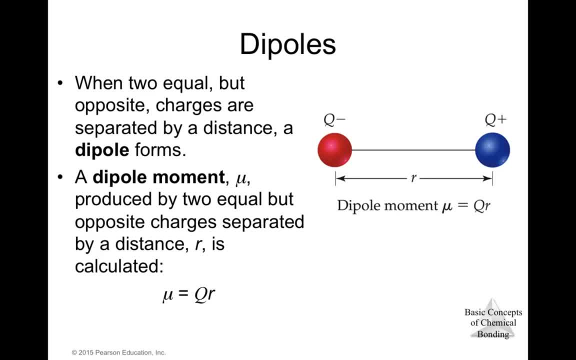 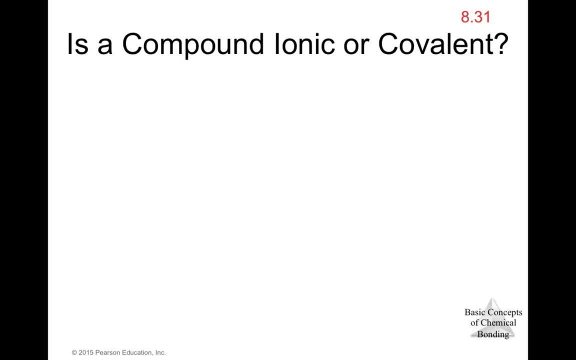 moment, the more polar the bone. so how do we measure the dipole moment? so how can we determine if a molecule is, or a compound is, ionic or is covalent? well, we have a few um hints that could help us to determine what type of compound is. the first one is the 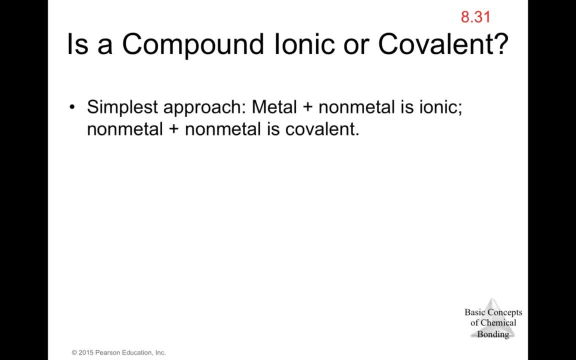 simpler approach. if you see a metal with a non-metal, you said that is an ionic. if you uh see a metal, a non-metal with a non-metal is a covalent. another way also is to determine the difference in electronegativity of the two atoms involved in that bond. that way we can. 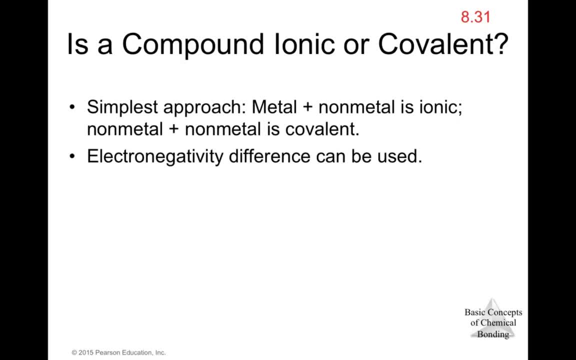 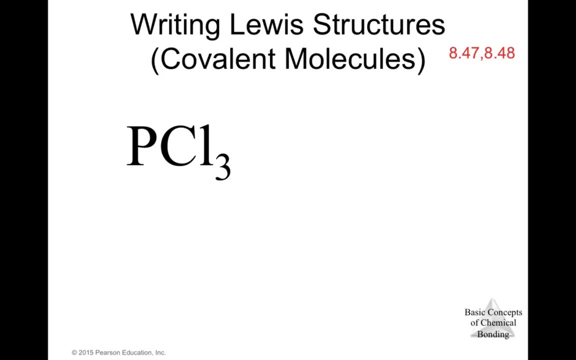 determine if that molecule could be also ionic or covalent. and the third way also is to look it up for the properties of the compound. for example, the lower the melting points, that means that that compound is a covalent one. now here we're going to learn how to write Lewis structures. 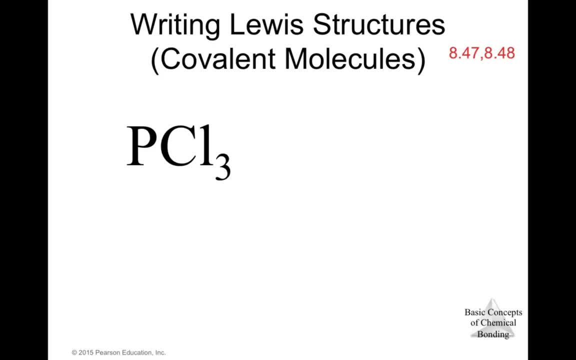 and these are just for the molecules. so first we need to sum the valence electrons from all atoms, taking into account overall charge. so here we have phosphorus and chlorine. so we have one phosphorus, phosphor. basically, a is from family five and chloride from family seven. so if, if this compound or 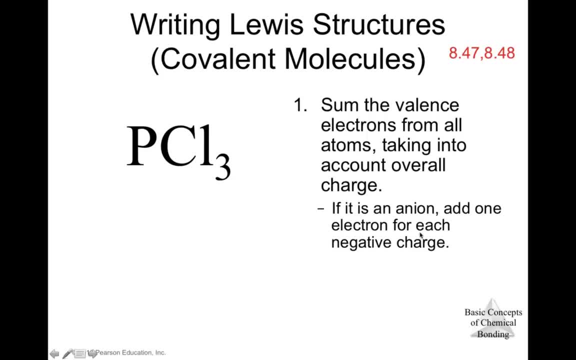 if we have a molecule that is a non-ion, we need to add an electron for each negative charge. if it's a cation, we need to subtract one electron for each positive charge. so here we have, as i mentioned, phosphorus from family five, chlorine, for family seven. we have three of 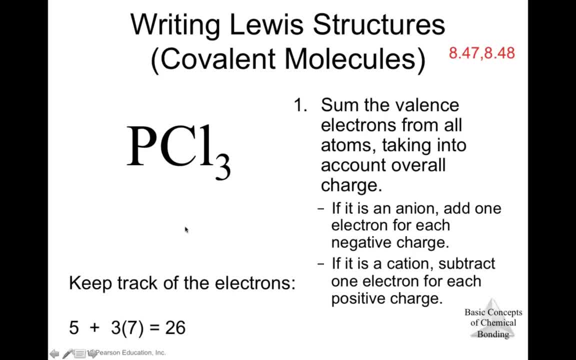 chlorine. so we multiply seven times three and because the seven is the family and that represent the valence electrons, okay, and uh, phosphorus is from family five, so it has five valence electrons, so at the end we're gonna have 26 electrons that we need to distribute around. 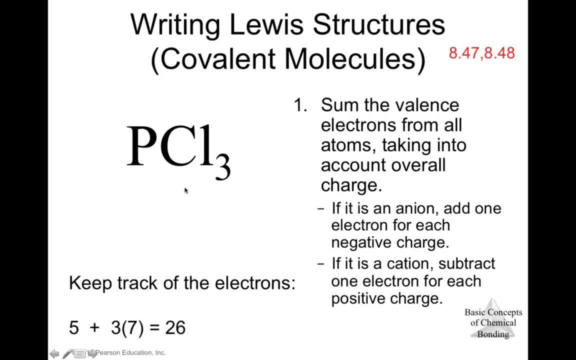 the molecule in a way that each of them has the complete, the octet rule. okay, and remember that in this case this is a neutral uh molecule, but maybe we have a polyatomic anion or cation that we need to determine also uh, the, the, the structure of that, or we want to write the loose structure, remember. 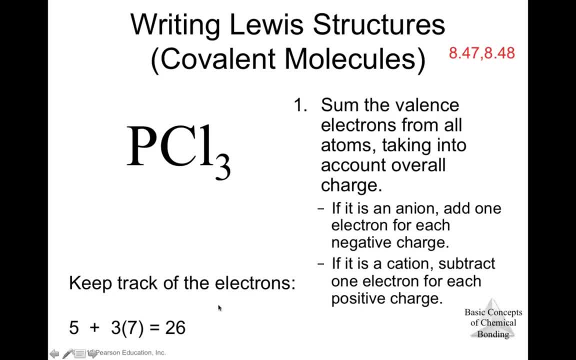 that, if that, if that ion is an anion, we need then to add one electron here. if it's a cation, we need to subtract. if it's just a container of a positive one, we need to add one electron. here we need to subtract just one electron. so for each electron that you add, you're going to add. 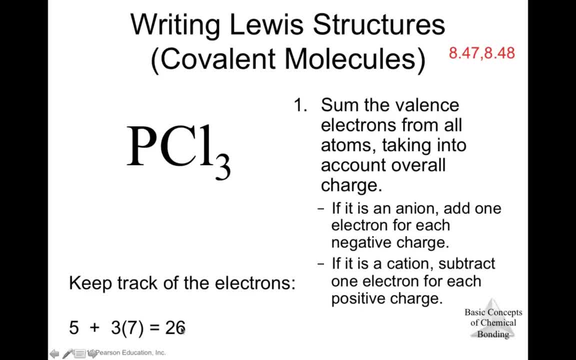 a number here. so if you add three electrons, so you may need to add three electrons at the total that you calculate initially for each family. okay, so if it's a neutral, just follow the group that they are and count just the valence electrons and that will be all the number of electrons. 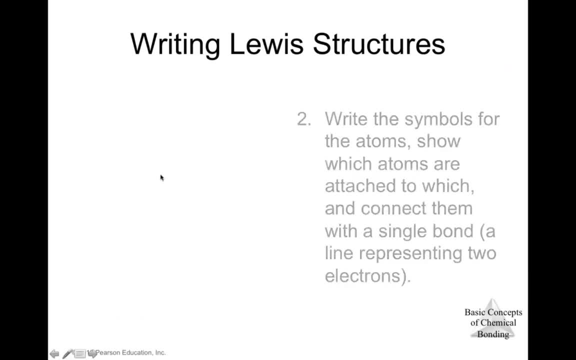 you need to distribute all around the molecule. so write the symbols for the atoms, show which atoms are attached to each and connect them, and it's with a single bond. so we're going to put first here the phosphorus in the middle, because it can create more bonds if you write a structure for the 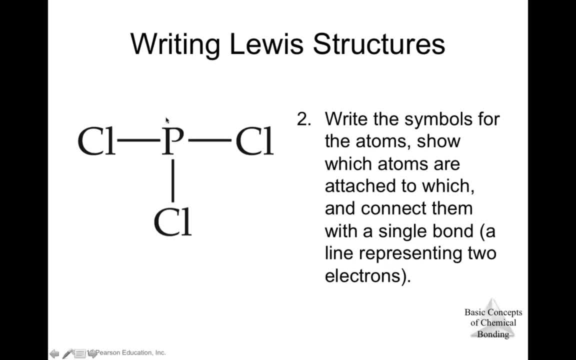 loo for the loose structure. just for phosphorus. you will see that you have an unpaired uh elect, a pair of electron, a long pair of electrons and three unpaired electrons. so those three unpaired can make bonds. you have three possibilities to create bonds and you can create bonds with chlorines. because it's seven, you will have three long pairs. 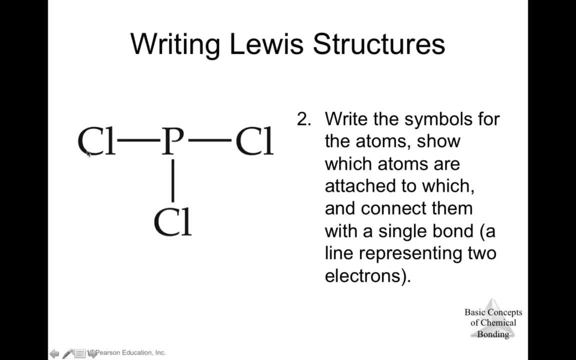 electrons and one individual electron. so that means that you can just create one bond with chlorine. so you're going to put in the middle the atom that can create more numbers of bonds. so that's why you put phosphorus in the middle and you're going to put one bond between them. 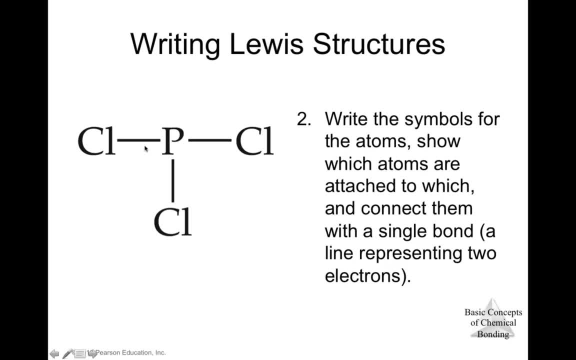 okay, and each one represent how many electrons each bond? each one represents two electrons that we mentioned before. okay, so keep track of the electrons. we have 26 at the beginning to start with, and we're going to subtract six that we use to create those three single bonds. okay, so now we have 20 that we need. 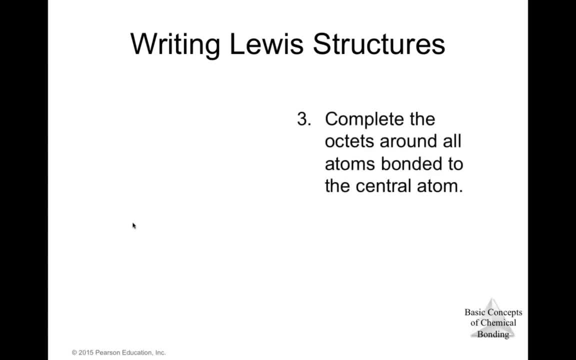 to distribute all around the molecule. so complete now the octet rules. the octa is around all the atoms bonded to the central atom. so here we have two, four, six and two. here we have eight, two, four, six. and here we have eight, two, four, six, and we have eight also here. so 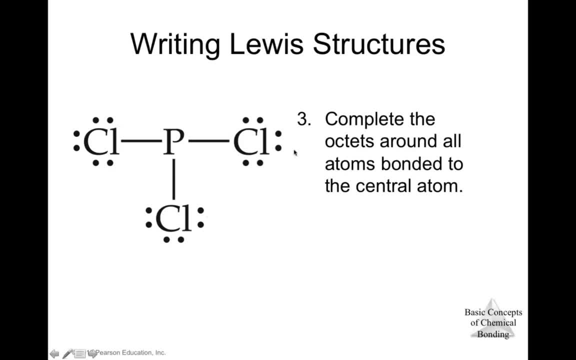 added one, two, three, four, five, six, seven, eight, nine a pair. so that means 18, uh, basically 18 electrons. so we have now 20 minus 18 is equal to two. so we have two left so we can add it in the molecule and we so we can see here that the phosphorus has just six electrons around it. so we 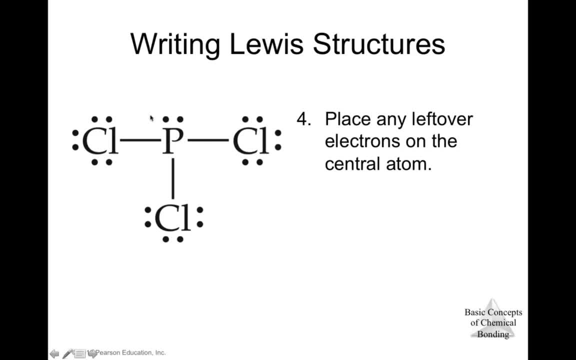 then can place those electron on the central atom, so in that way it also complete the octet for that atom. so here we just need to look for the uh balance electrons in a way that we can uh draw this, uh blue structures, and now two minus two basically is equals zero, so we use all the elect. 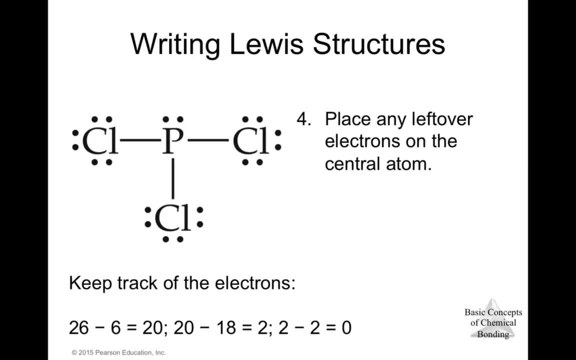 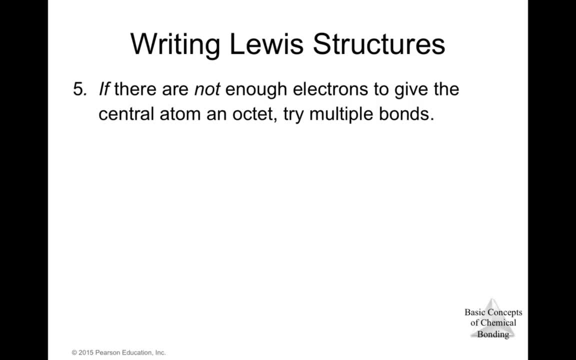 possible balance electron, balance electrons, uh, to draw this structure. now, if there are not enough electrons to give the central atom a knock, that if you use all the electrons and you still see that central atom is not, it doesn't have yet the octet, you need to use multiple bonds. so in this case we 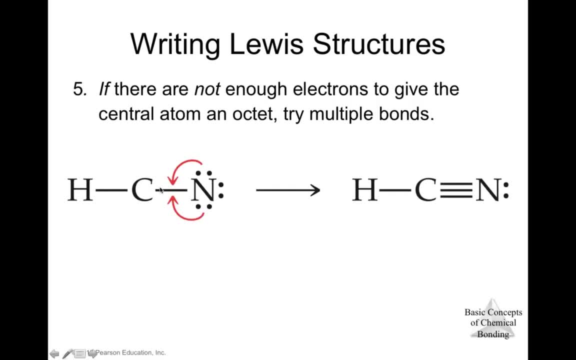 have this: h hc end is a molecule and this is the initial structure, the loose structure. but we can see here that for hydrogen, remember that hydrogen needs to have just two electrons around it and that's their, that, this, that's their octet. okay, because it's an exception for the rule, because 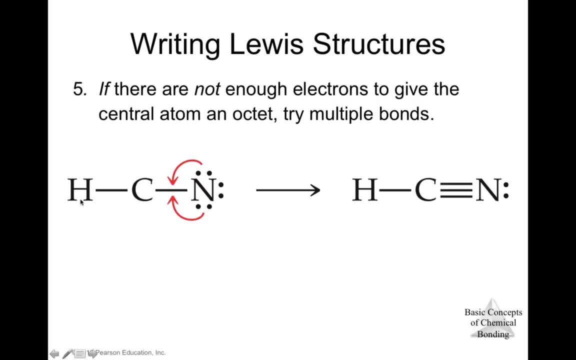 it doesn't have, it does it. it's just filled that one s orbital, so it will be okay with two electrons. so with hydrogen we just need to uh two electrons around it. so we have here that is complete, that octet rule exception. and with nitrogen, we have here eight electrons around. 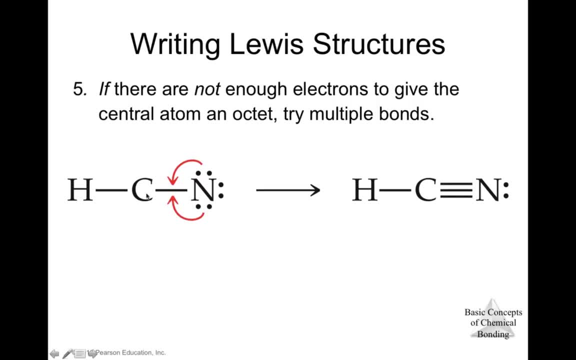 but with carbon we just have four. so we need to start to create double bonds between the carbon and the nitrogen, multiple bonds, so we can use one of the lone pairs of the nitrogen and create a double. remember that each bond represent two electrons, so we from these two electrons, we 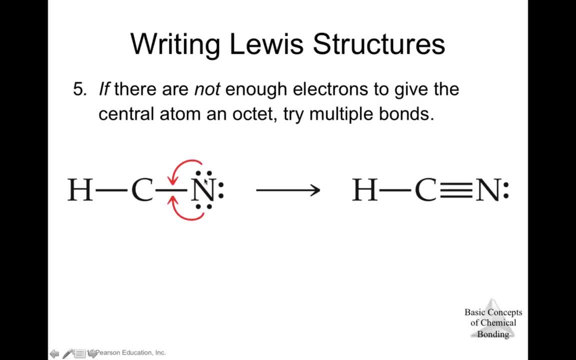 one bond between these two atoms and also with these two electrons we can create one bond between those two atoms. so now we have one, two, four, six, eight electrons are on carbon, all of them. you can see that they are sharing the electrons between those three, two atoms. 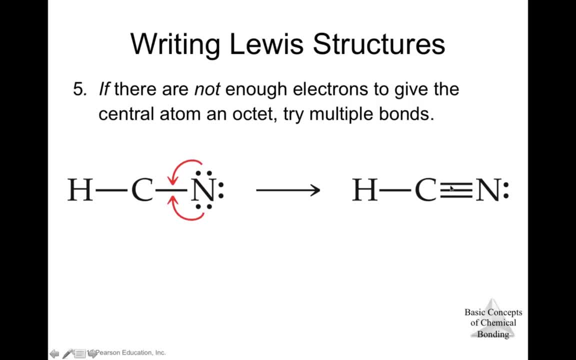 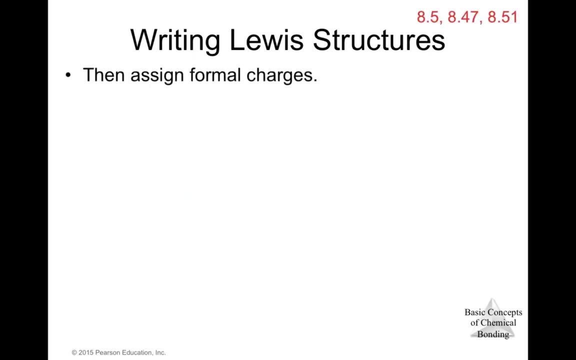 and here the nitrogen has six in the triple bond because we have two electrons for each bond plus two here, so now we have the octet around the nitrogen as well as with the carbon. also, sometimes we need to assign formal charges because we have ions sometimes. so we the former. 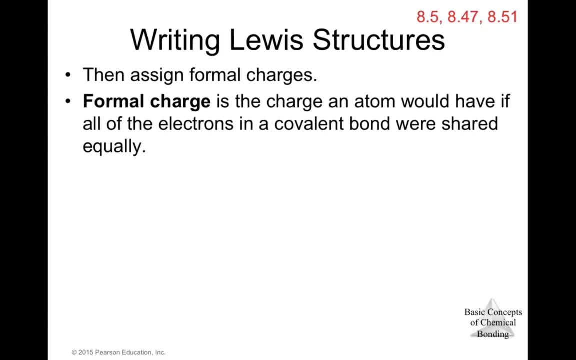 charge is the charge an atom would have if all the electrons in a covalent bond were shared equally. so former charge is going to be equal to the valence electrons minus half of the bonding electrons, minus all non-bonding electrons. this is one formula. we can create all different kind of formula but this. 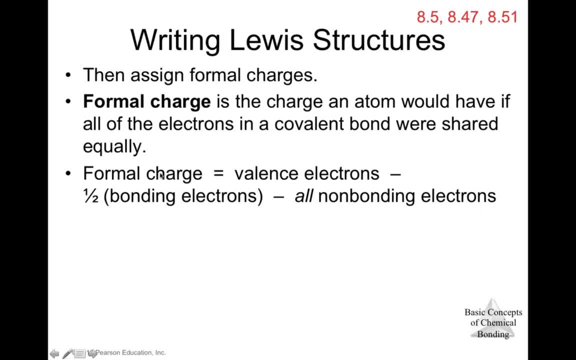 one is the uh. that's going to give us also the formal chart. but this one is using the valence electrons, the total valence electron minus half of the bonding electrons, minus all non-bonding electrons. so what that means here we have, for example, for carbon dioxide writing as this way: 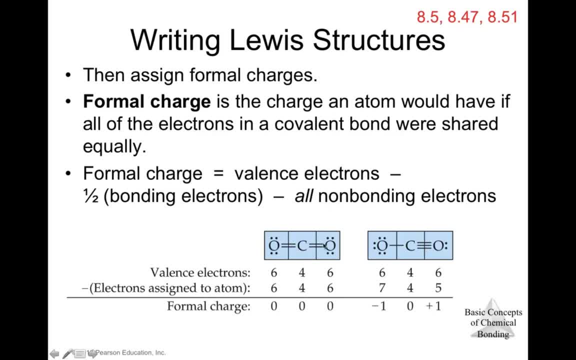 carbon, double bond, double bond and oxygen and oxygen here, uh, we can see that we have the octet. for this oxygen, we have two, four and here we have four more. remember that we have two electrons for each bond, so we have eight electrons around this oxygen. same way with the carbon: we have four bonds around it, so each bond is represented with. 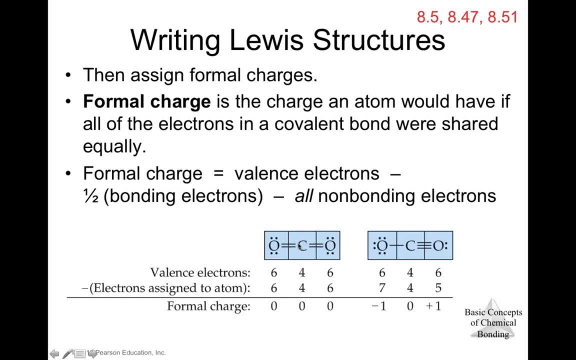 two electrons. we have eight um electrons here and here we have, uh, basically also eight electrons. okay, so we have the octet for each of them. so the valence electrons for oxygen- oxygen Oxygen- is from family 6, so it's 6.. Carbon is from family 4, so the valence electron is 4.. 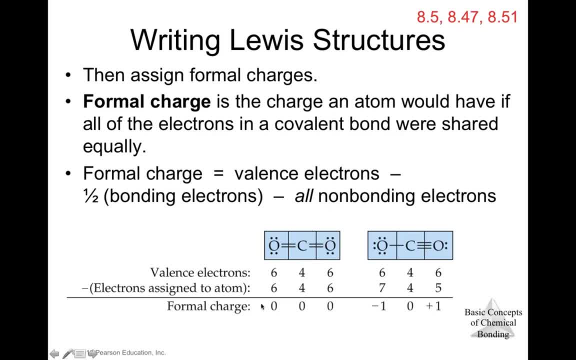 And oxygen is also 6, so we have here the valence electrons. Now we need to subtract the electrons assigned atoms. So we have for half of the bonding electrons. we have 2 from here. We have 4 that are doing a bond, but we're going to use half of them. 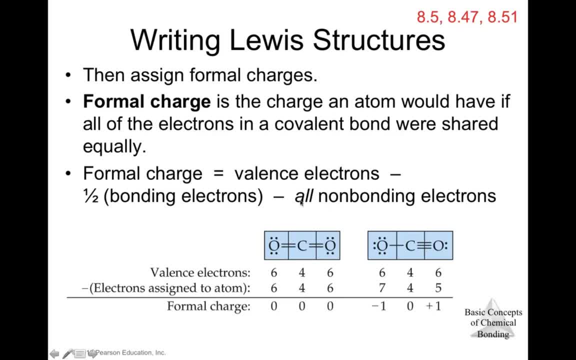 So instead of 4, we're going to use 2.. 2 plus all non-bonding electrons. so non-bonding, we have 1, 2, 3, 4.. That means that 4 and 2 is 6, so 6 minus 6 is 0.. 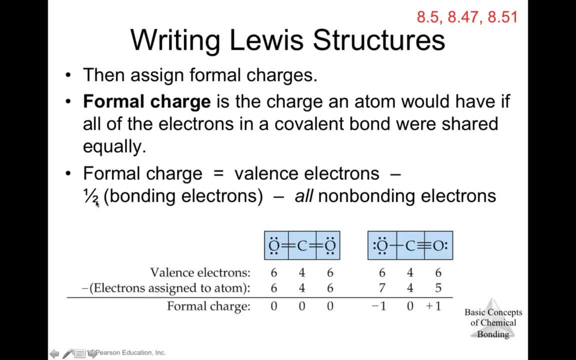 For carbon and this carbon specifically, half of the bonding electrons. we have 8 bonding electrons around that carbon, so half of it is 4.. It's going to be 4 minus 4 is going to be equal to 0.. 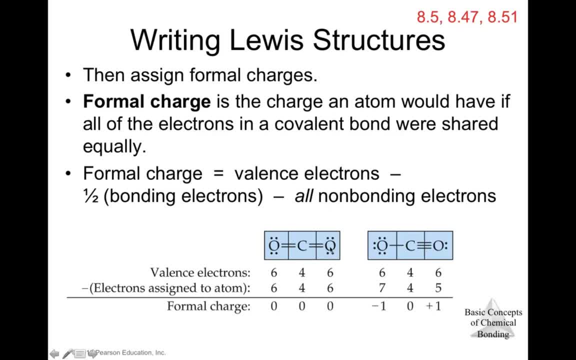 And in this oxygen the same thing. it's valence electron 6, half bonding electrons. We have 4 bonding electrons, so half is going to be 2.. And all non-bonding electrons 1,, 2,, 3,, 4- for this oxygen. 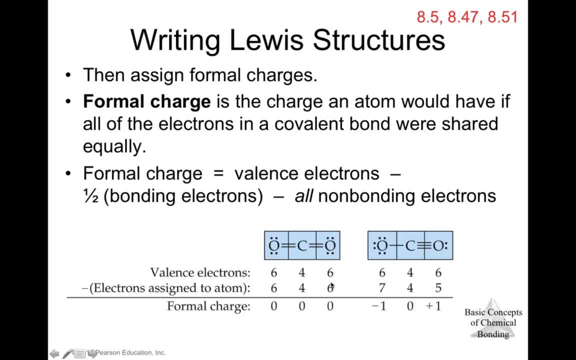 so it's going to be 4 plus 2 is going to be 6.. That is this 6, so 6 minus 6 is equal to 0.. So the formal charge for all these atoms is going to be 0.. 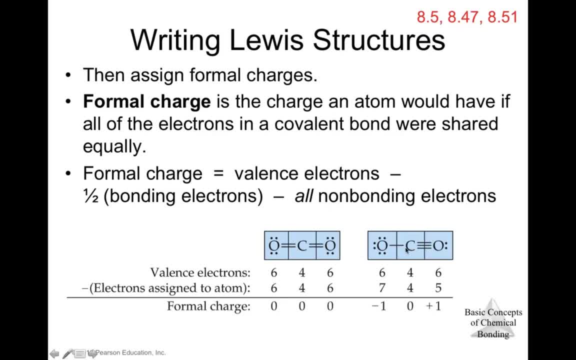 Now, in this other structure that we can see here, it's also 4 carbon dioxide, but it's a little bit different because instead of 2 double bonds, we're going to have 1 single bond between this carbon and oxygen, a triple bond between this oxygen and carbon. 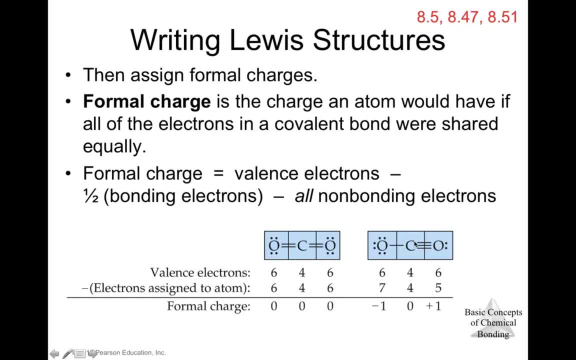 And even though it's a different arrangement of the electrons, you still have 8 electrons around this oxygen. We have 2, 4, 6, and these 2 are 8.. So you have the octet rule with this one. 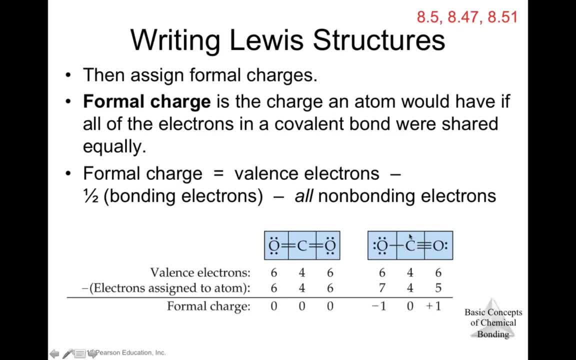 And with this carbon you have 2,, 4,, 6,, 8.. We have also 8 electrons around this carbon. Remember, each bond has 2 electrons, So we have 4 bonds in this carbon. We have 8 electrons around this carbon. 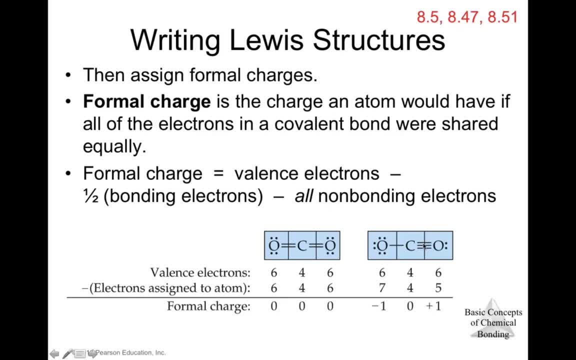 And with this oxygen we have 3 bonds, So we have 6 electrons, plus these 2, we have 8.. So now we're going to look for how many electrons are assigned for each atom. So in this case, by using this part of the formula, 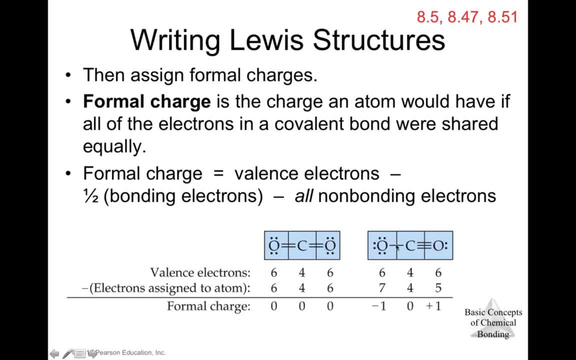 we need to look for half of the bonding electrons. We have 2 bonding electrons here, So that means that half of these- 2 is 1, plus all non-bonding electrons. For this oxygen we have 2,, 4,, 6 plus 1 is 7.. 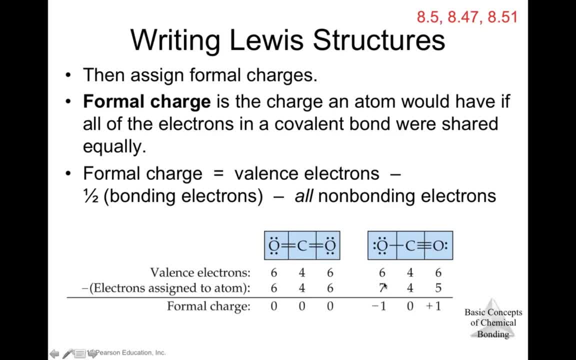 So that's why here we have a 7. The electrons are assigned for this atom, For carbon. basically, we have half of bonding electrons. We have just bonding electrons in this carbon We have 8. Half of them is 4.. 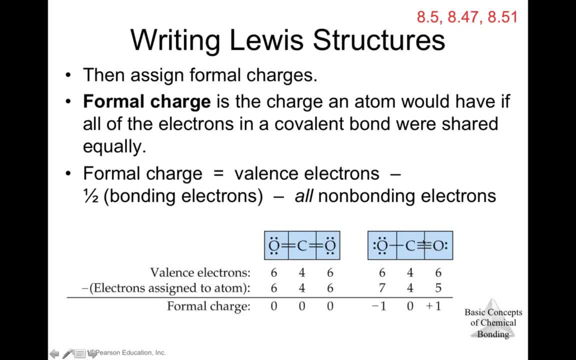 And for this oxygen we have half of this. 6 electrons is 3. And we have 2 non-bonding electrons. That means that we have 5.. So when we subtract this, it's 6 minus 7.. It's going to be minus 1.. 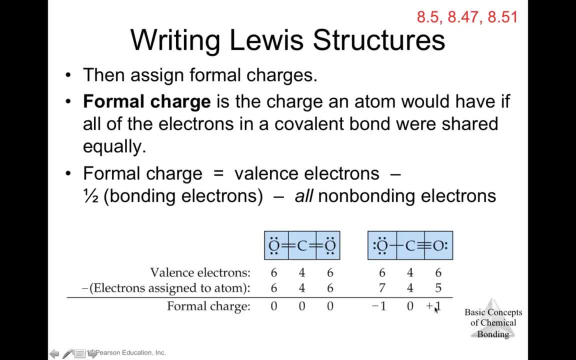 6 plus 5 is going to be 6 minus 5.. It's going to be plus 1.. So that means that this oxygen will have a charge of minus 1., A formal charge of minus 1. And this one will have a formal charge of positive 1.. 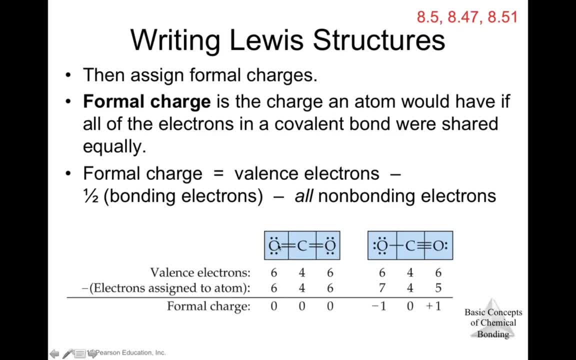 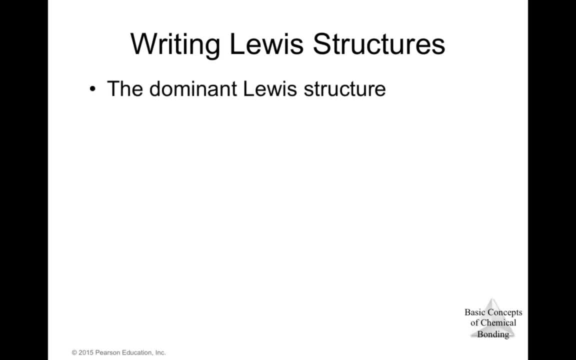 While in this arrangement of electrons all of this has a 0 formal charge. So we saw that we have 2 different Lewis structures in the slide before. Which one is going to be the dominant? It's the one in which the atoms have formal charge. 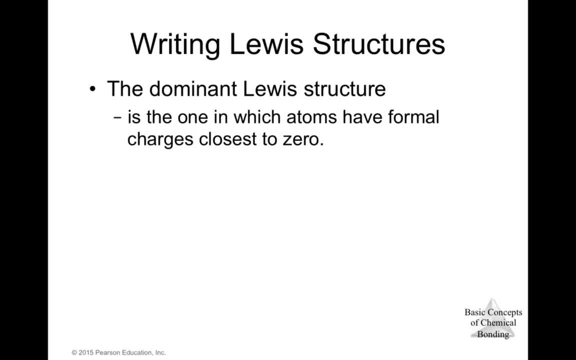 The one in which the charges are closest to 0 or 0. As was in the first one in the left, Puts a negative formal charge on the most electronegative atom also. So in this case, for example, here we have N and Cs. 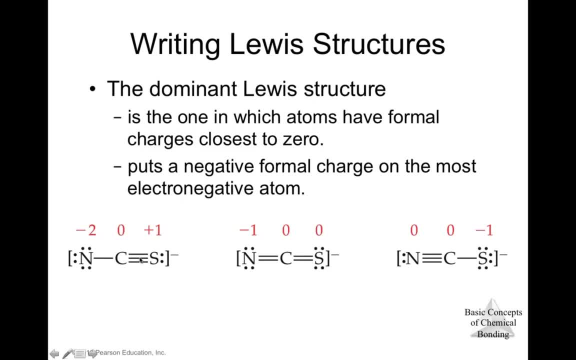 We have 3 different Lewis structures And all of them are correct in the perspective of the octet rule. But what about the charges? We see here that the most dominant structure, 3, are correct, But there's going to be just one that is dominant. 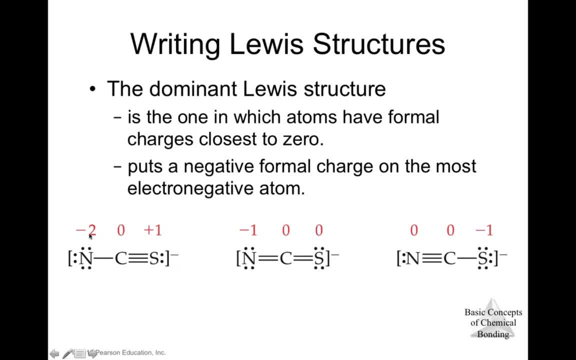 This one is the less dominant because it has numbers larger than 0 or different from 0. And this too, So here we have just 1 and 1 here. Here we have 2 atoms with different charges or a charge different from 0.. 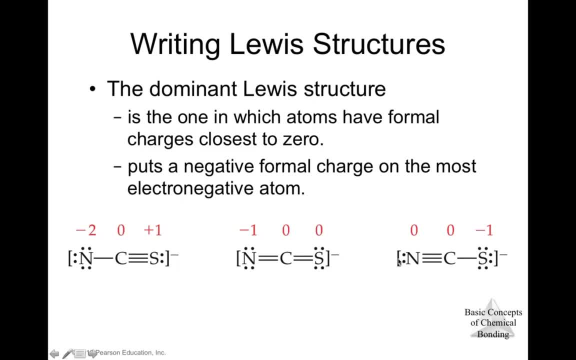 So this one is not the most dominant. So we have this one and this one. They have a minus 1 and 0, 0 formal charges. They have a 0, 0 and minus 1 charges. So that means that we have basically the same distribution. 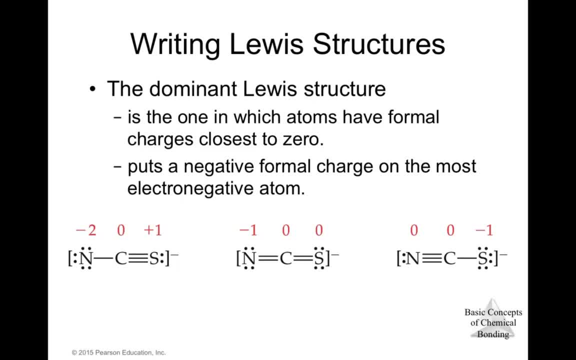 In the formal charges. But we need to have that negative in the most electronegative atom. That in this case is going to be sulfur. So this is the most dominant structure for the Lewis structures. These are correct, but this is going to be also the dominant Lewis structure for N, C, S. 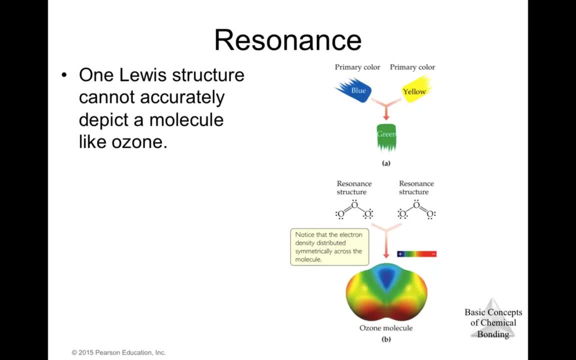 So one Lewis structure cannot accurately depict a molecule like ozone. We use multiple structures, known as resonance structure, to describe the molecule. This is ozone here And we can see that sometimes we have a multiple bond, double bond between these two oxygens And sometimes we have the multiple bond between these two oxygens. 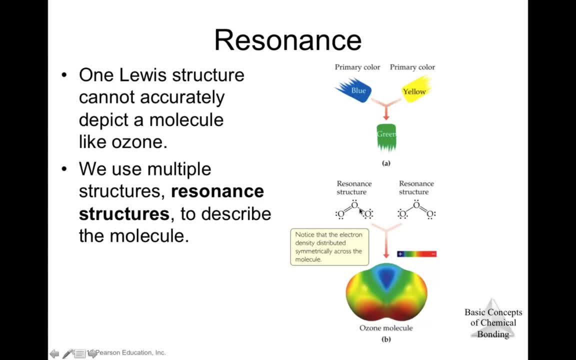 That means that the electrons have been moving around this area. We have the double bond here and then we have the double bond here. That's a resonance. It's called resonance structures. So this is the resonance structure of this structure. That is, the distribution of the electrons across the molecule. 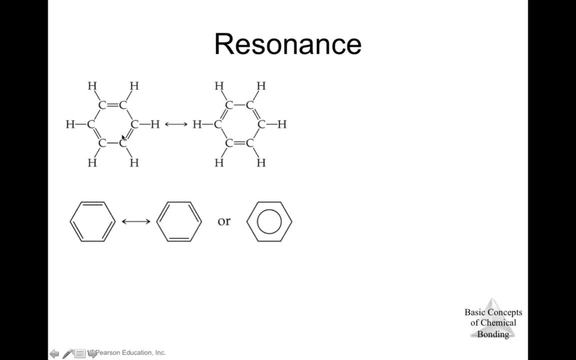 And here we have one example of benzene. This is a benzene ring. We have the double bond between these two carbons, Between these two carbons and these two carbons, And we can see that we can move those double bonds in a way that, instead of being here, 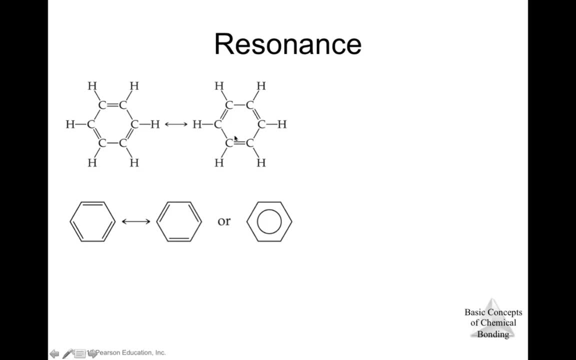 Now they are going to be in other places, They do a resonance structure. This is also the same representation, but without showing the atoms. But this represents the carbons And we don't write hydrogens in this type of representation, But we still have the double bond between these two carbons. 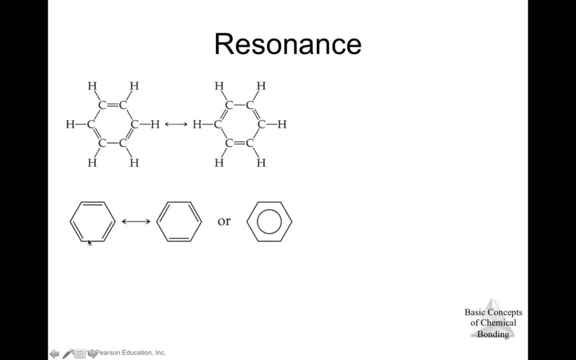 Single bond between these two carbons, Double bond between these two carbons, Single bond between these two carbons. You can see that you have double bond, single bond, double bond, single bond, double bond, single bond, As well as here. 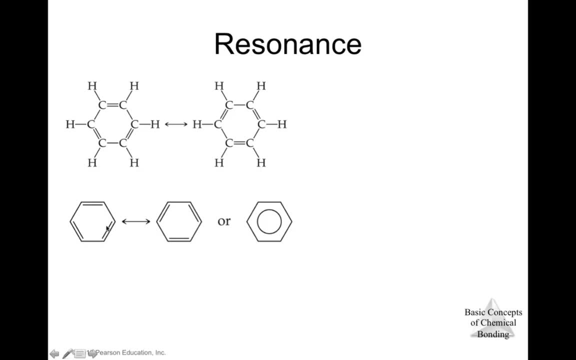 Now this double bond moves to this point. This one moves between these two carbons And this one moves between these two carbons And we have this structure And this is happening really, really fast. So we can represent this as this ring with a circle inside. 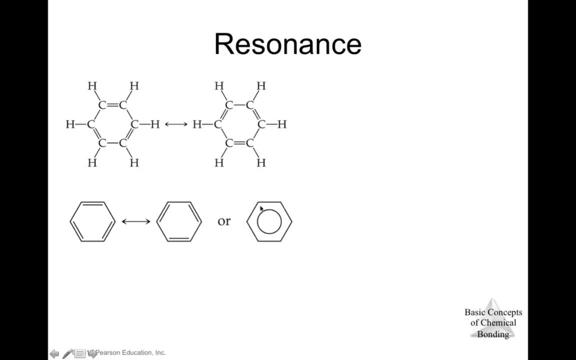 Which represents resonance. It means that the electrons are moving all around the molecule, Because we can see that we can move this to here To create this double bond. This double bond can move to here To create this one. So they are moving all around the molecule. 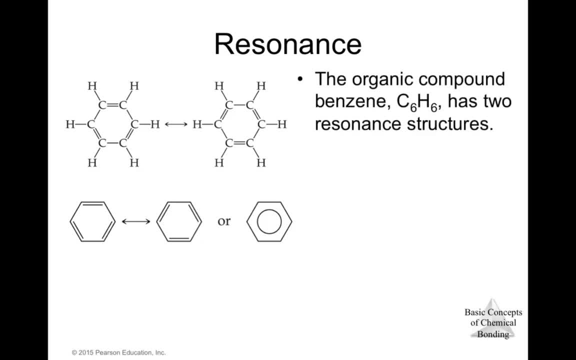 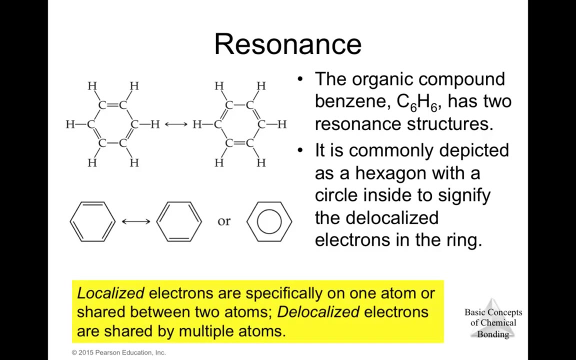 So this is the organic compound, This is the benzene C6H6. That has those two resonance structure And it is commonly depicted as a high hexagon With a circle inside to signify the localized electrons in the ring. So localized electrons are specifically on one atom. 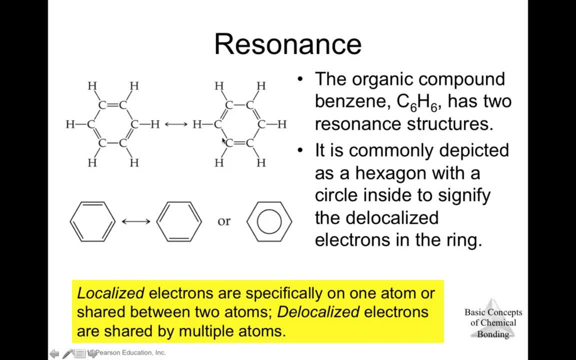 Or shared between two atoms. So this one is the localized electrons. They are always between these two carbons, But this one of this is going to be always between these two carbons, But the other one is going to be moving all around the molecule. 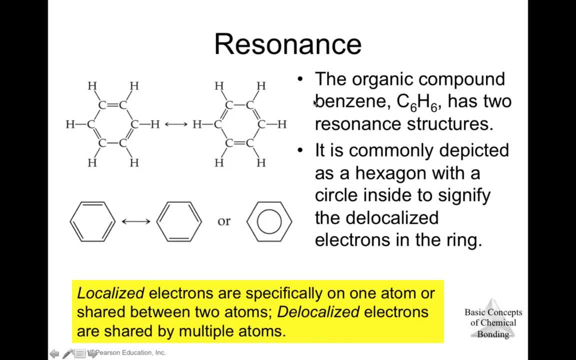 So we are going to have the localized electrons That are shared by multiple atoms. So those that create those multiple bonds are the localized, Because they are moving all around the molecule. While, for example, this one is localized, These two electrons are always between these two, hydrogen and carbon. 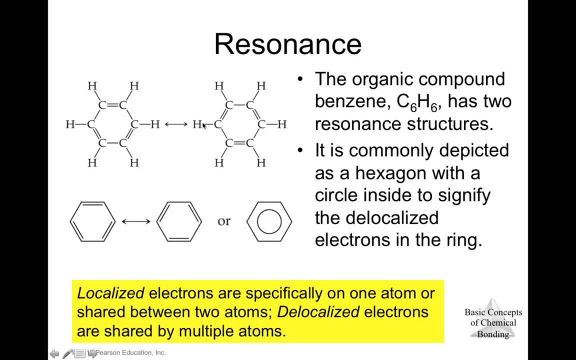 These two atoms, These electrons are localized, As well as this one, As well as one of these two double bonds. One of these bonds is going to be moving all the way around the molecule, But the other one is going to stay doing the bond between these two carbons. 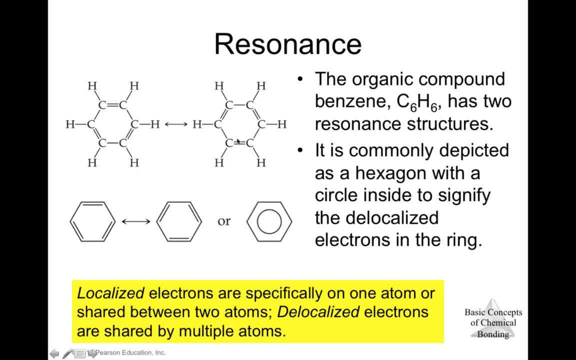 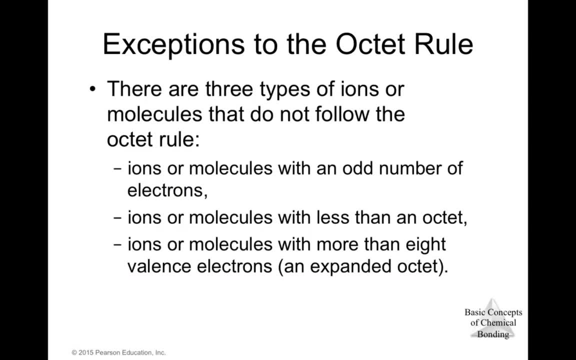 So one of these is going to be localized And the other electrons are going to be delocalized. Now there are some exceptions for the octet rule. There are three types of ions Or molecules that do not follow the octet rules. 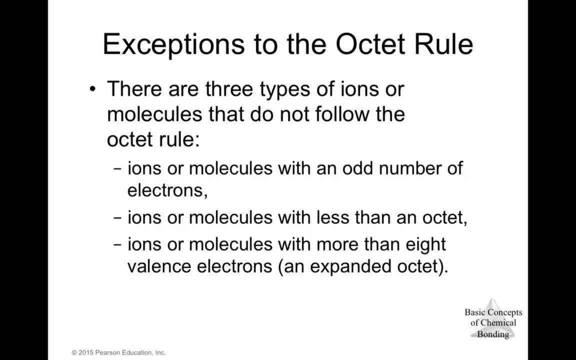 First one. Ions are molecules with an odd number of electrons. They are also known as radicals. Ions are molecules with less than an octet, And ions are molecules with more than eight balanced electrons. That is known as the expanded octet. 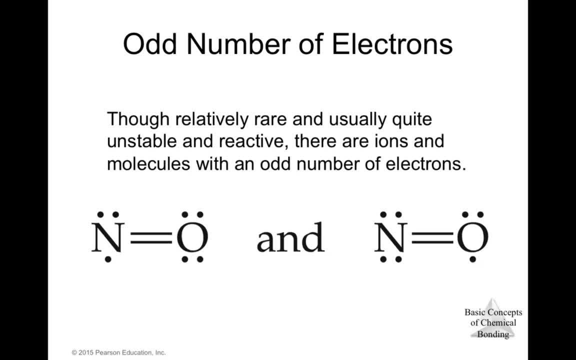 So here we have an example of the odd number of electrons. Though relatively rare and usually quite unstable and reactive, There are ions and molecules with an odd number of electrons. Here we have the nitrogen with just one electron. here. That means that we are going to have five electrons around this nitrogen. 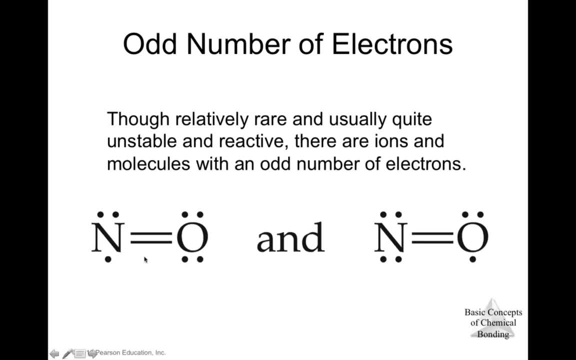 And when we do a resonance structure, Or basically a resonance structure of this one, We can create here also a radical. And we have around this oxygen just five electrons, And this is an exception for the octet rule. The other one is when we have fewer than eight electrons. 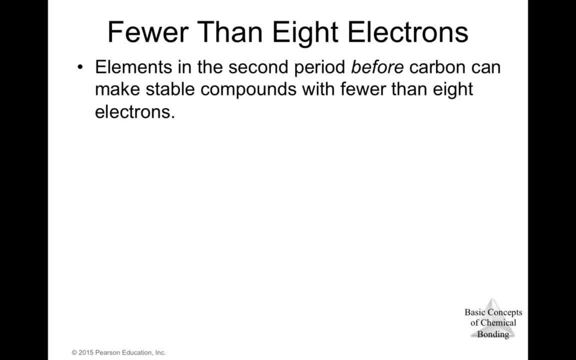 Elements in the second period before carbon can make stable compounds With fewer than eight electrons, as we saw with hydrogen. Okay, And also, for example, boron BF3.. BF3: given boron a full octet place a negative charge on the boron. 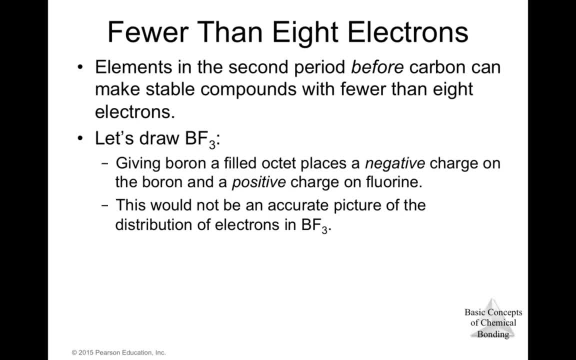 And a positive charge on fluorine. This would not be accurate picture for distribution of electrons in BF3.. So we have here the boron And we can write this structure, Lewis structure for BF3. Where each fluorine has basically eight electrons. 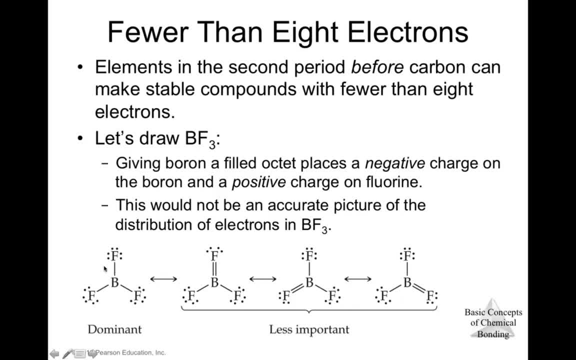 So it has the octet complete, While boron still has is just have six. Okay, So we can rewrite to make boron like the octet. to complete that octet, We can do a draw a double bond. We can use one of this pair of electrons to create that double bond. 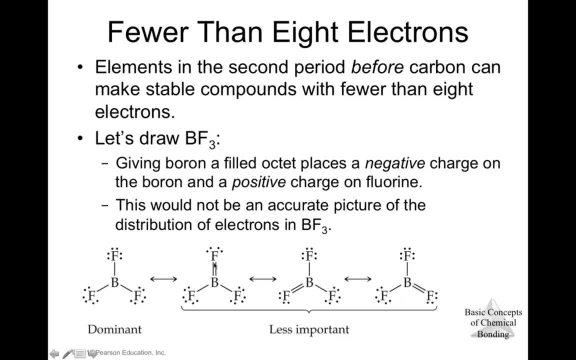 But if we do this, Each fluorine here with a double bond, each fluorine is going to be a partial positive And we know that fluorine is the highest element with the highest electronegativity. So they love electrons, They want to have electrons. 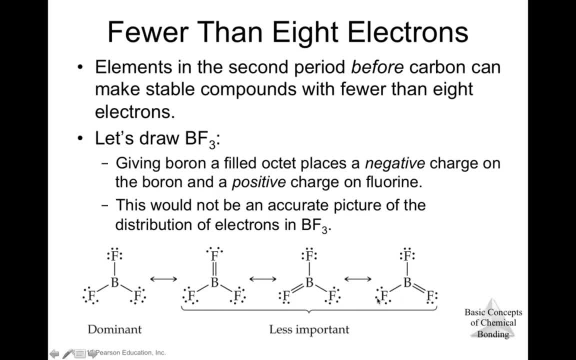 They don't want to get rid of electrons, So that's why these are less important, Even though they are correctly drawn. But because of that difference in charge, We're going to have a positive charge here And a negative charge here, While here we're not going to have any charges. 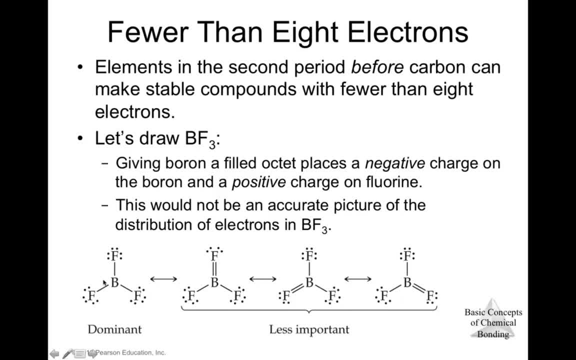 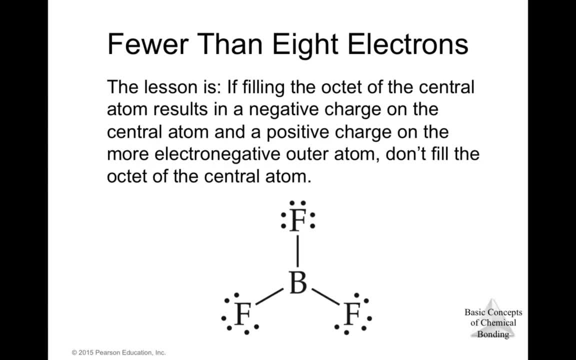 So that's why this one is the dominant structure. The lesson is that if filling the octet of the central atom results in a negative charge on the central atom And a positive charge on the more electronegative other atom, Don't fill the octet of the central atom. 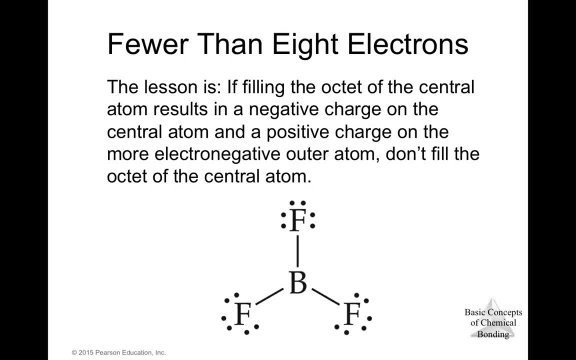 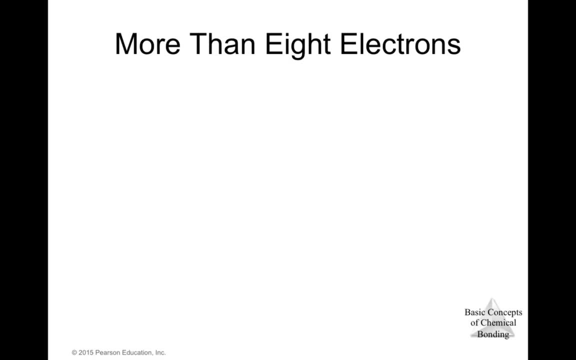 It's not going to be favorable. So that's why, in this case, boron is really happy that we just have less than 8 electrons, Even though it's not an octet, And we also have examples or exceptions with atoms that could have more than 8 electrons. 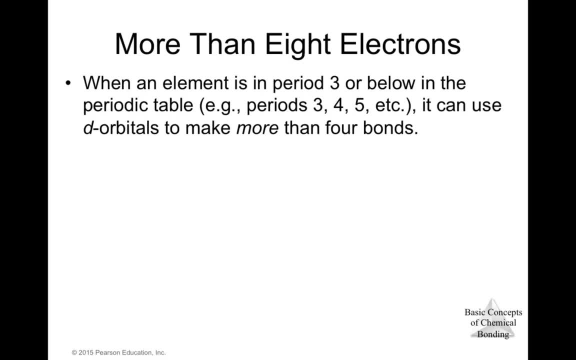 When an element is in the period 3 or below in the periodic table, Period 4 or 5.. It can use the orbitals to make more than 4 bonds. The example is PF5.. And also the phosphate, So we can have here the PF5.. 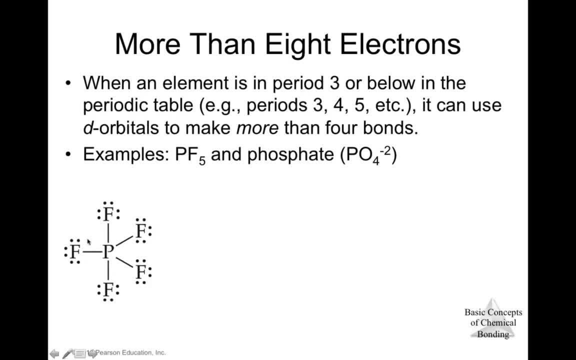 We have the phosphorus in the middle And around all the phosphorus we have 10 electrons. It has more than the octet But because it has the orbitals available, They can use those orbitals to To accept those electrons from the fluorine. 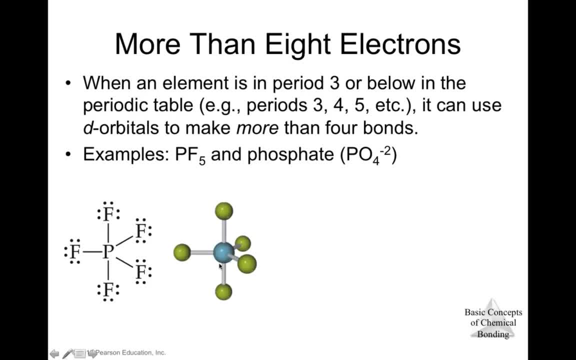 This is basically another kind of 3 dimensional structure for PF5.. And here we have the phosphate. The phosphate here has basically 8 electrons around And also has a complete octet, as well as the oxygen. But, as we can see, here we have 5 charges. 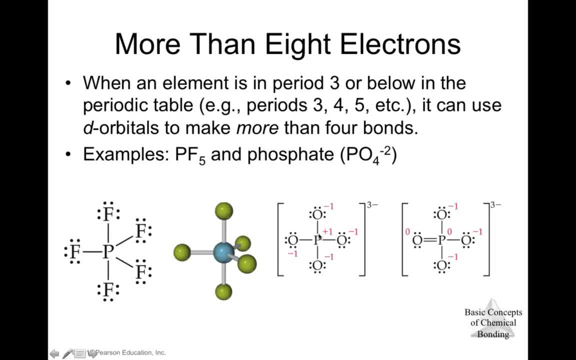 A complete of 5 charges: 4 negative 1 and 1 positive 1.. While, if we can create a double bond between an oxygen and a phosphorus, Now we're just going to have just 3 charges. So we are looking for. 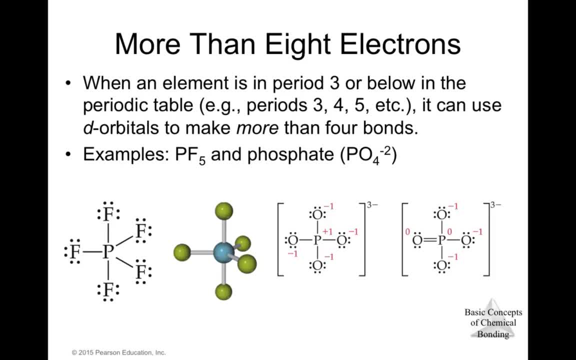 To look for the structure that has the less number of charges in each atom. So that's why, even though this is a correct one, It completes all the octet. But because phosphorus has the orbitals also available, We can put those electrons in those orbitals. 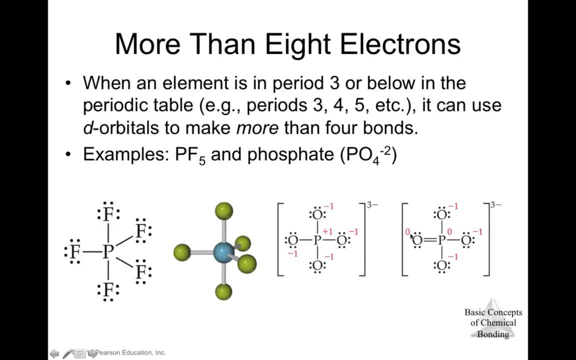 And by that way decrease the charges, The partial charges In the molecule. So we can have just 3 instead of 5. And even though we're going to still have The ions going to be minus 3.. Okay, But, 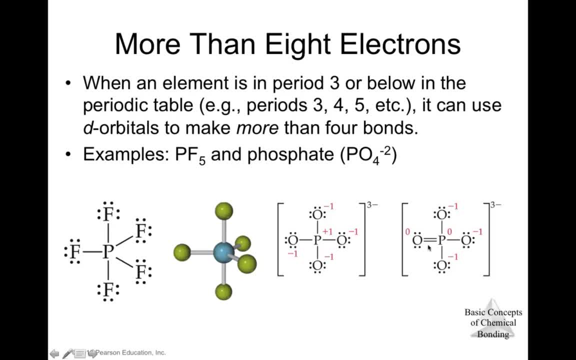 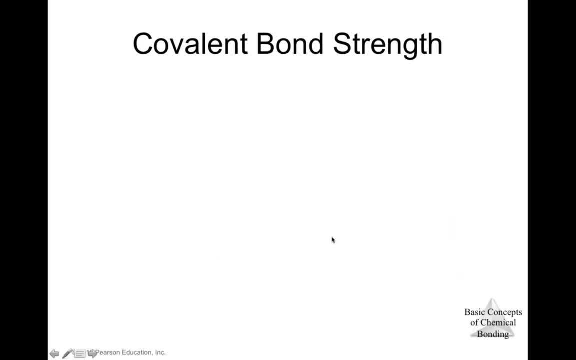 In this case, We're going to have less distribution of charges in the molecule, So this one is predominant over this one. Now let's talk about the covalent bond strength. Most simply, the strength of a bond Is measured by determining how much energy is required to break the bond. 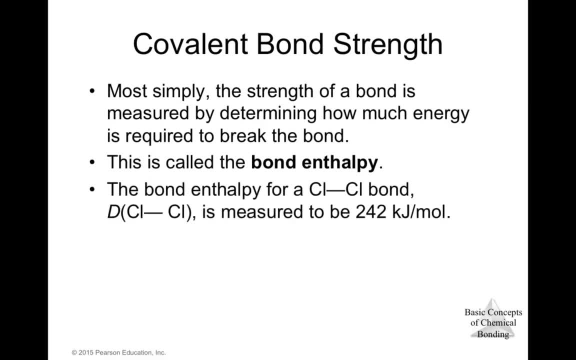 This is called the bond enthalpy. So the bond enthalpy for chloride bonds, ClCl, is measured to be 242 kilojoules per mole. We write out reaction for breaking one mole of this of those bonds, So we can break. 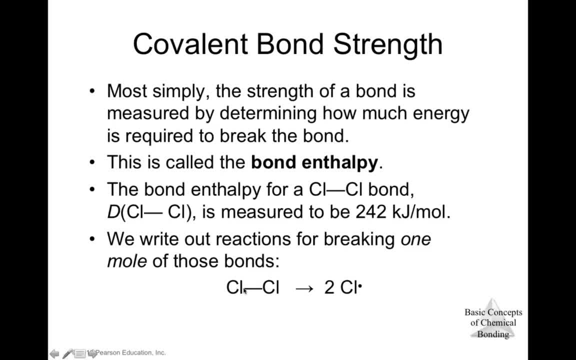 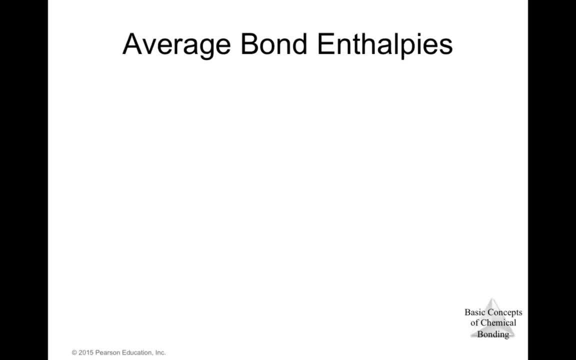 The bond by saying that we're going to distribute These two electrons, going to give one electron for each side. So we're going to have two radicals of chlorine. And now we talk about the Average bond. Enthalpies are positive Because bond breaking is an endothermic process. 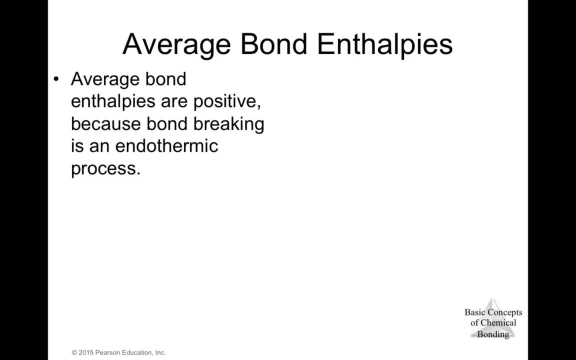 You need to add energy. So that's why the enthalpy is going to be positive, So you can break those Bonds. Note that these are averages over many different compounds. Not every bond in nature For a pair of atom has exactly the same bond energy. 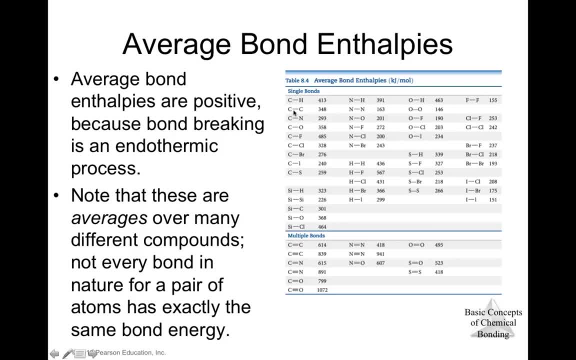 So That means that not all of the carbon-carbon single bond. You need to add 348 kilojoules. Sometimes you need to add a little bit more or a little bit less. This is just an average, Because Those bonds could be in different molecules. 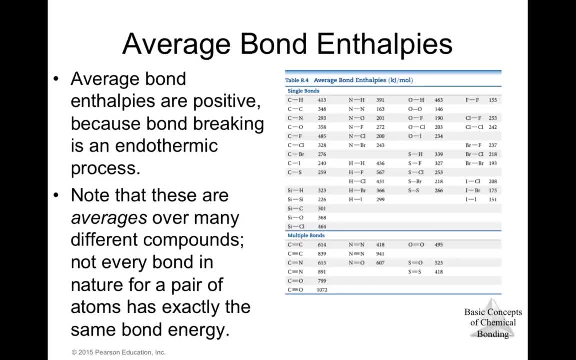 And because of different molecules They can have a little bit different In the strength of that bond, But the average is going to be, for example, 348.. So what do you think is going to be The average bond enthalpy for a double bond of carbon-carbon? 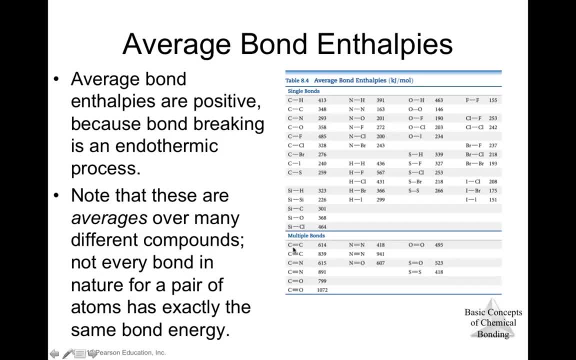 Is it going to be higher or lower? It's going to be higher Because now we need to break two bonds between those carbons. So that's what we can see here: That the average bond enthalpy for the double bond is 614 kilojoules per mole. 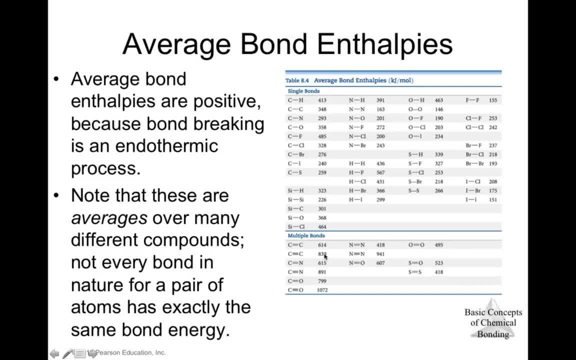 While for the triple bond is 839 kilojoules per mole, So it's higher The multiplicity of those bonds. You're going to have also a higher average of bond enthalpy. You need more energy to break those multiple bonds. 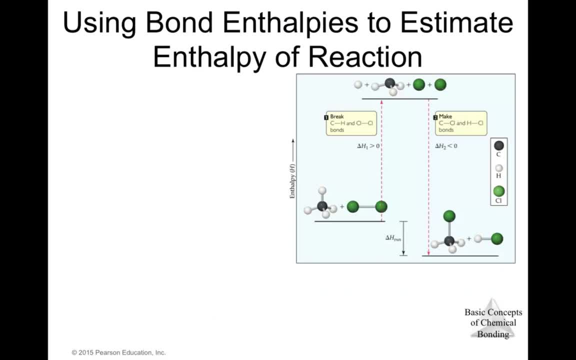 So using bond enthalpy to estimate the enthalpy of a reaction. Now we know that the enthalpy of a reaction Is the energy that may be required or be released When you're doing a reaction, So we can calculate that energy of the reaction. 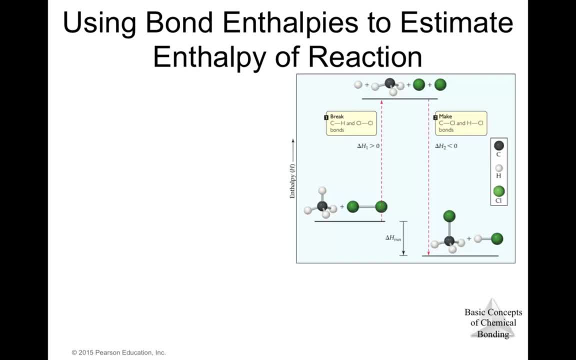 By knowing The enthalpy of the bonds. So one way to estimate the delta H for a reaction Is to use the bond enthalpies of bonds broken And the new bonds form. So energy is added to break bonds And release when making bonds. 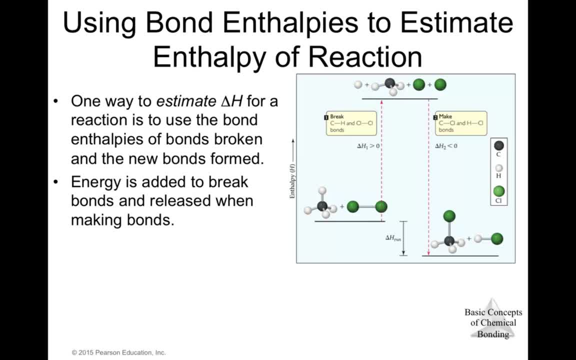 So we're going to always We're going to add energy So we can broke those bonds. But when we create bonds We're going to release energy. So in other words, The delta H of the reaction is going to be equal. 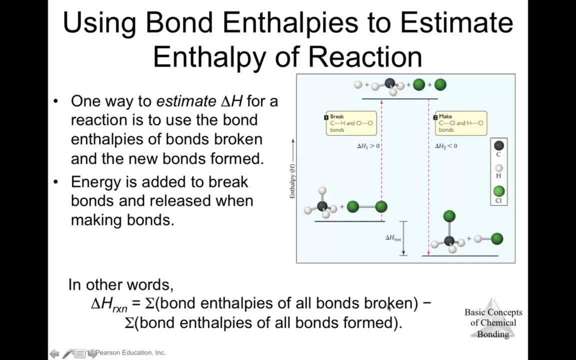 To the sum of the bond enthalpy For all bonds broken, Minus the sum of the bond enthalpies Of all bonds form. Okay, so here, For example, we have methane And we have chlorine. So here we are. 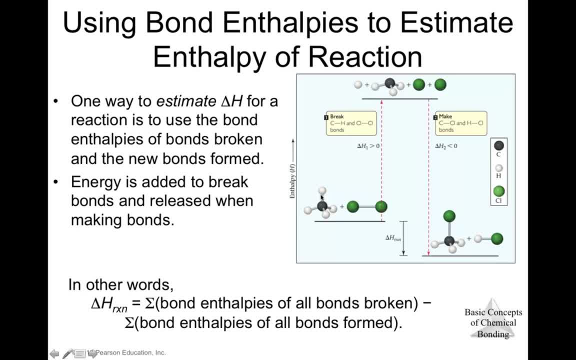 So we can see, at this point We broke one bond Between a carbon and a hydrogen. So that's why we have a hydrogen here And the CH3 now Is. before was CH4. But now we remove one hydrogen, We have the CH3. 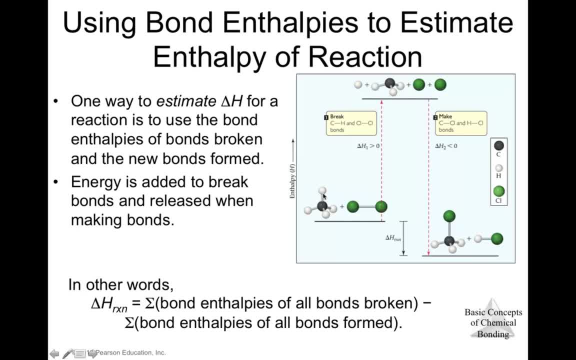 To do that, we need to add energy. We need that energy to break this bond. The same thing happens with the chlorine, With the CO2.. We need to create this: two radicals here. We need to break this bond And we need to add energy. 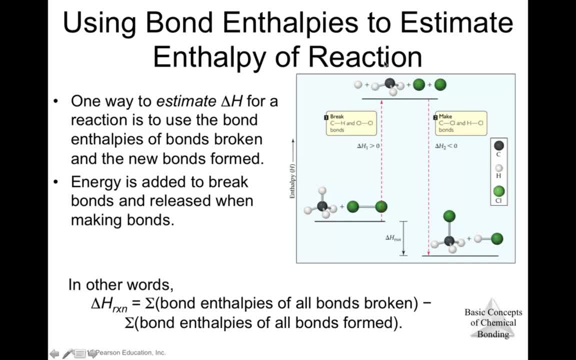 Now, when we create the bonds Between this chlorine and this hydrogen And this chlorine and this carbon, Energy is released And we can see here that Actually the products Has less energy than the reactants. So that means that That was an exothermic kind of reaction. 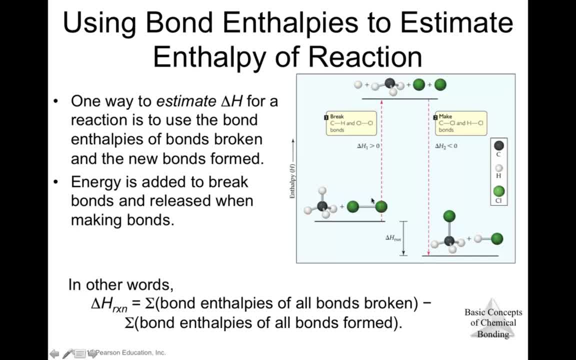 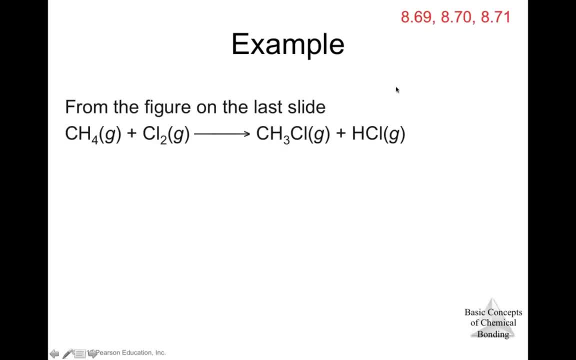 Because it released more energy Than the way that you used to broke The bonds to create this radicals. So from the figure on the last slide, We have that This methane and the chlorine Producing the chlorine, Methane and the HCl. 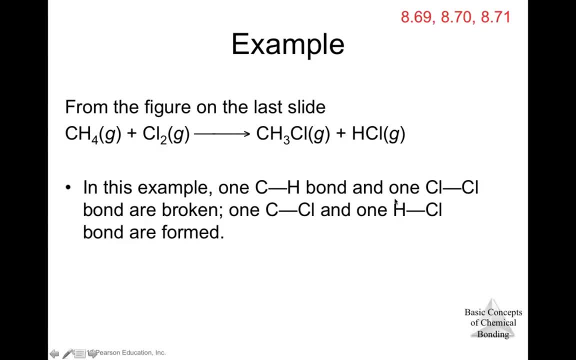 In this example, One carbon hydrogen bond And one chlorine CLC bond are broken- One from here and one from here- And one carbon chlorine and one HCl bonds are formed. We formed with one of this chlorine Bond to one of the carbon. 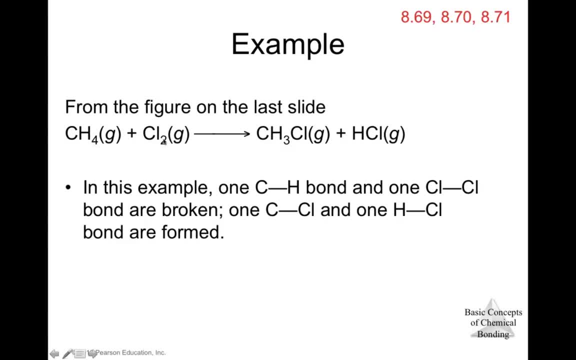 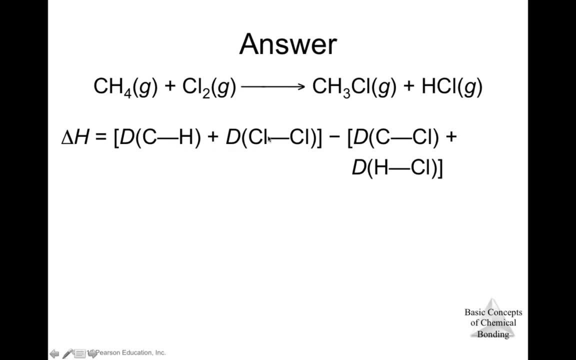 And the hydrogen was released Bond with the other chlorine. So now We need to look for the Enthalpy for each of the bonds. Okay, And that's in the table. Here we have 413 kJ And here we have 242 kJ. 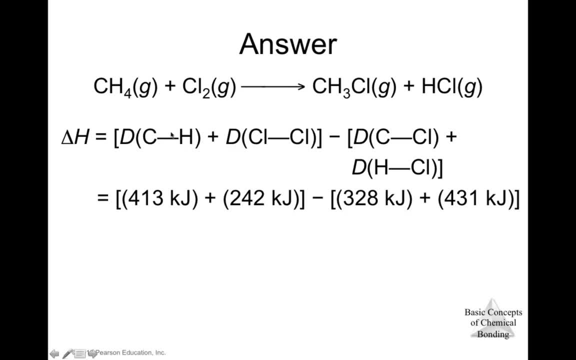 For the chlorine-chlorine bonds. So this is the energy that is required To break those bonds, Minus Enthalpy for each of the chlorine that was formed. So it's going to be 328 kJ For carbon-chlorine. 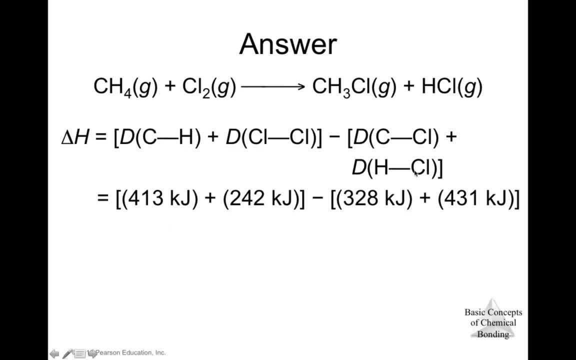 And 431 kJ For hydrogen-chlorine, And that means that we have 655 kJ Minus 759 kJ, And we see here that The reaction is an exothermic one. It releases energy. This is: 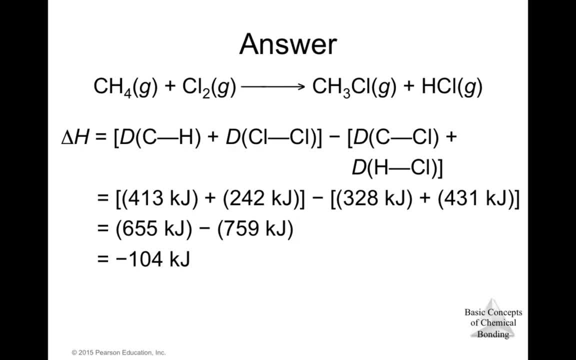 Agree with the figure that we saw before, Where we saw that the products Has lower energy than the reactant And in this way We can measure the enthalpy Of a reaction. Remember that will be the sum Of the enthalpies of the. 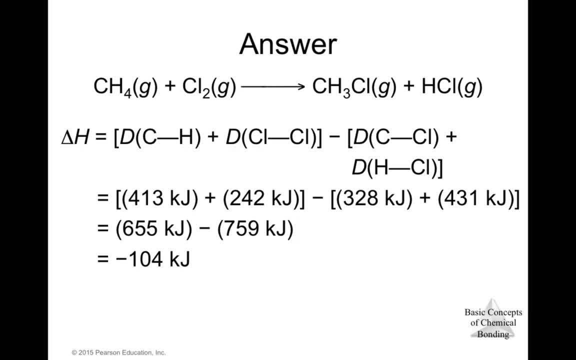 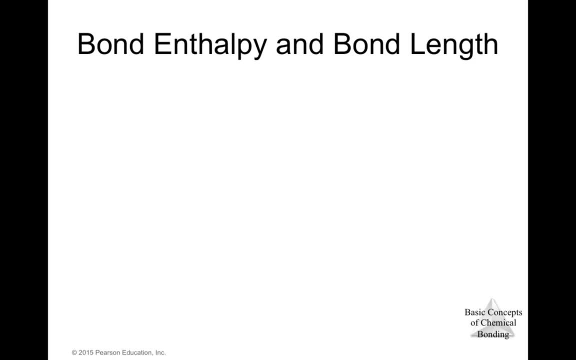 Broken bonds Minus the enthalpy of the formed bonds. Also we can relate The bond enthalpy And the bond length. We can also measure an average bond length For different bond types As the number of bonds between the two atoms increases.